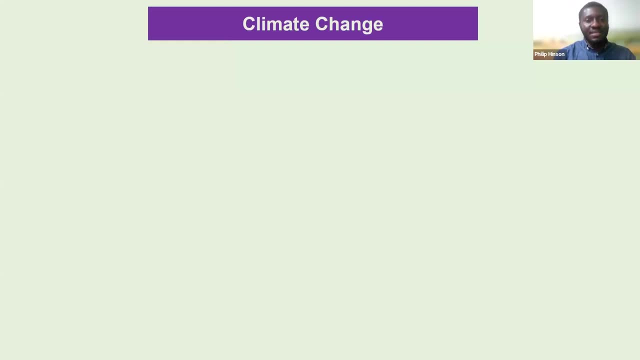 questions you may have. So, believe it or not, climate change poses the greatest threat to humanity and therefore demands immediate action, or immediate and coordinated actions by all individuals and by all countries. Climate change can simply be defined as a long-term shift in temperature and weather patterns. Since 1800s, human activities have been the main driver of 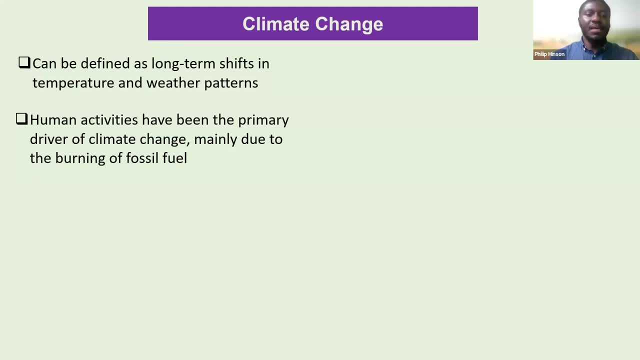 climate change, primarily due to the burning of fossil fuel, And the consequence of climate change is more evident now than ever before. As I speak to you now, I'm in Pennsylvania and we are having our fair share of the wildfire smoke from the Canadian wildfires, If you are. 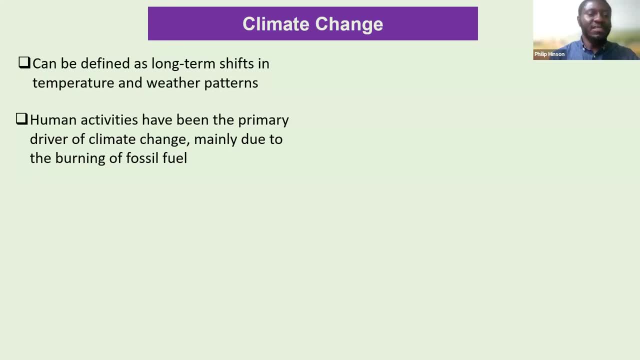 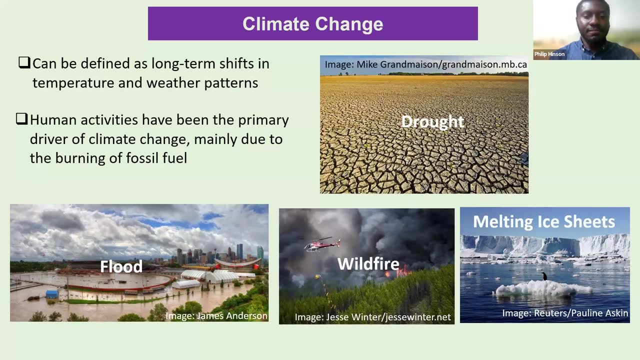 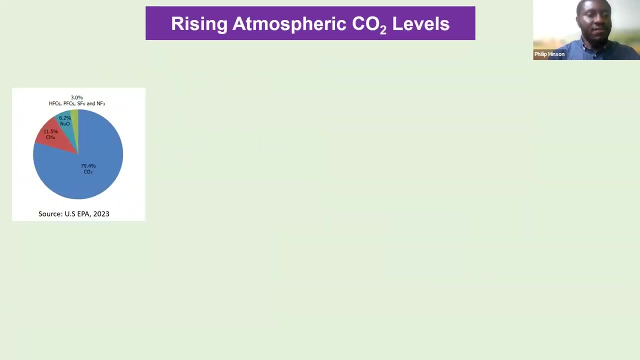 somewhere on the East Coast. you might or you may have experienced this already. So the effects of climate change include severe droughts, flooding, severe wildfires, melting ice sheets, rising sea levels, ocean acidification and many, many more. We know that there are lots of. 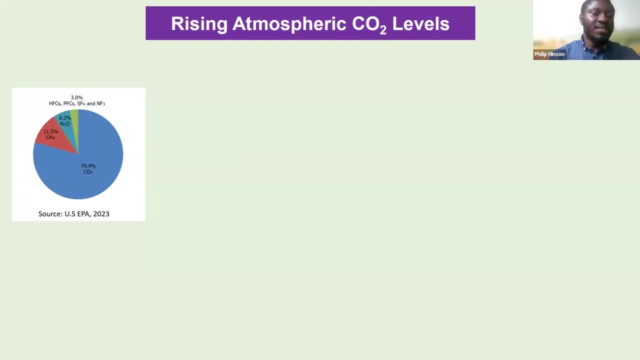 greenhouse gases in the atmosphere: carbon dioxide, methane, nitrous oxide, chlorophyll carbons and many other fluorinated gases, But by far the largest carbon-contributor to climate change is carbon dioxide, Our most abundant greenhouse gas in the atmosphere, accounting for nearly 80% of the total greenhouse gas emissions in the US In 2021, and this is according to the EPA. So you can say that carbon dioxide, or atmospheric carbon dioxide, is the primary cause of climate change. with carbon dioxide and необходiantいう. 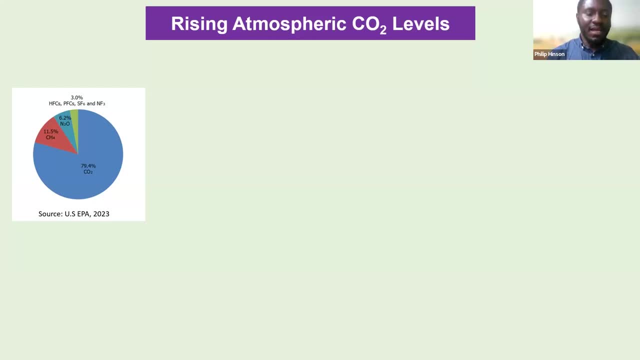 andclip escol— And, as you can see from this graph, the level of atmospheric carbon dioxide is increasing, but it is not only increasing. it is increasing at a much faster rate than before. So, for example, when the National Oceanic and Atmospheric Administration, or NOAA, started measuring atmospheric carbon dioxide in 1957, the rate of increase was about 0.5 ppm per year during the first 10 years. 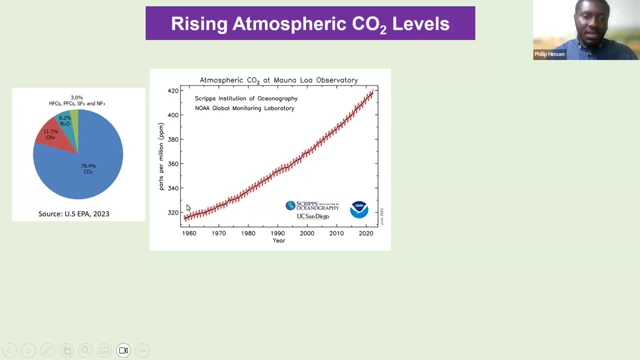 So that is evidence. you can see from this slope that we have relative mild slope. But in the last few decades, or in the last two decades, the rate of increase in carbon dioxide is about 2.3 ppm per year. This is a very disturbing or worrying statistic of facts. 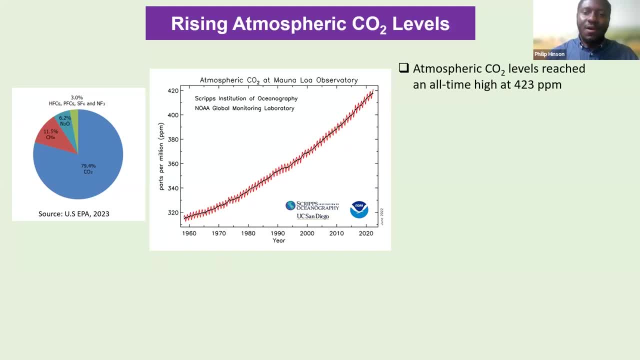 Speaking about disturbing stats of facts. did you know that on April 7th of this year, atmospheric carbon dioxide levels reached an all time high at 423 ppm? This is the highest level ever recorded in human history. So in my early 30s and in my lifetime, atmospheric carbon dioxide levels increased by more than 60 ppm. 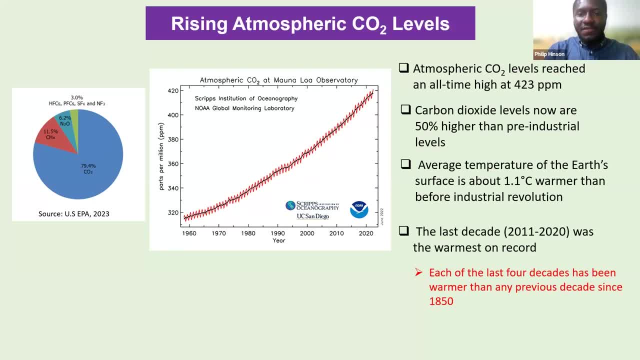 So the carbon dioxide levels are now 50% higher than before. So the carbon dioxide levels are now 50% higher than before. So the carbon dioxide levels are now 50% higher than before, higher than pre-industrial levels and the average temperature of the Earth's surface. 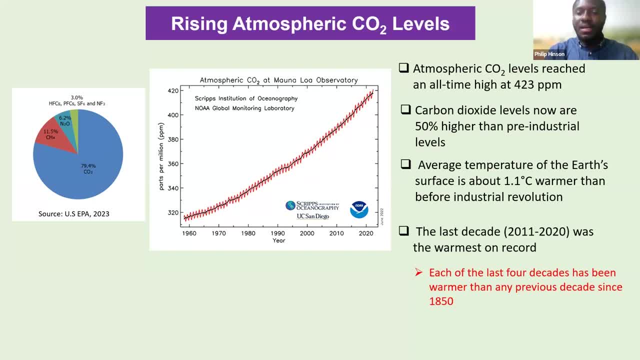 is about 1.1 degrees Celsius warmer than before industrial revolution, And we know that there is a strong correlation or relationship between rising atmospheric carbon dioxide levels and global temperatures. So the last decade, which is from 2011 to 2020, was the warmest on record. 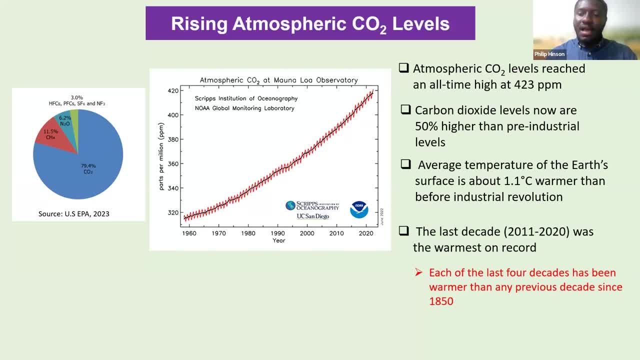 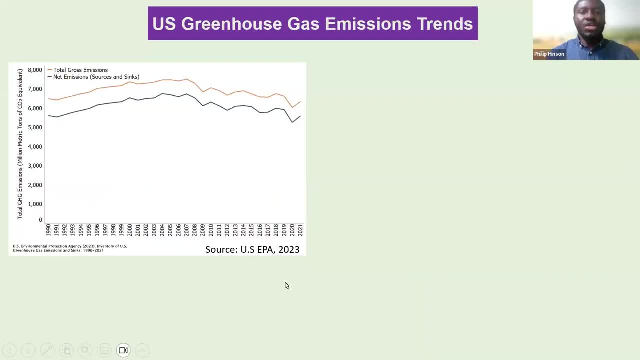 And each of the last four decades have been warmer than any previous decade since 1850.. This graph shows US greenhouse gas emissions over the years. The rusty orange line represents total greenhouse gas emission and that represents the total amount of greenhouse gas produced. 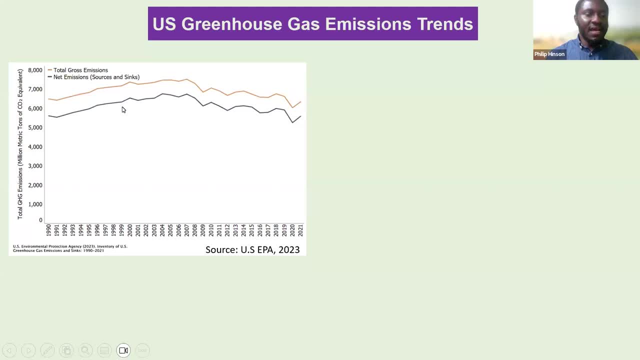 or released into the atmosphere. The dark gray line represents net emission, which is the difference between the total greenhouse gas, or the total amount of greenhouse gas produced or released into the atmosphere, and the total greenhouse gas emissions removed from the atmosphere. So the difference between these lines represents, or gives you an indication of, the total amount. 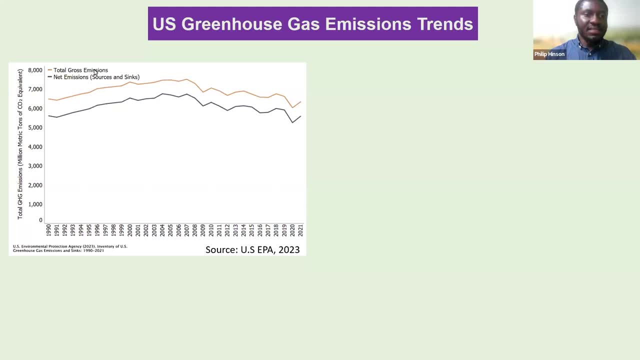 of greenhouse gas removed from the atmosphere And, as you can see from this graph, there hasn't been much improvement in the total amount of greenhouse gas removed from the atmosphere. So this tells us that we have work to do. We need to make this gap. 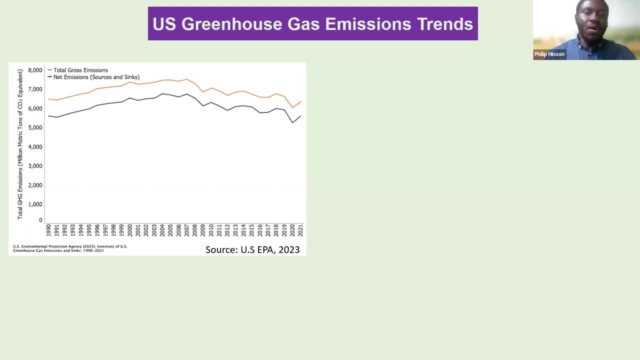 We need to make this gap. We need to make this gap wider. We need to remove more carbon dioxide, or greenhouse gases, from the atmosphere. So since 1990, the total greenhouse gas emission has decreased by about 2%. The dip you see in this total greenhouse gas emission in 2020 was as a result of the impact. 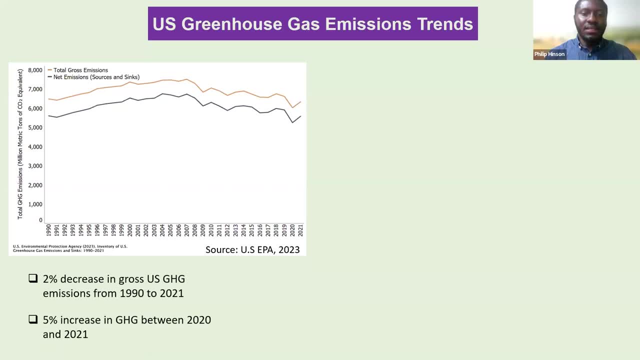 of COVID-19.. The impact of COVID-19: that has impacted travels and economic activities, But, as you can see from the graph, right after economic activities, after lockdown and economic activities started booming, the rates or the increase from 2020 to 2021 is now 5%. 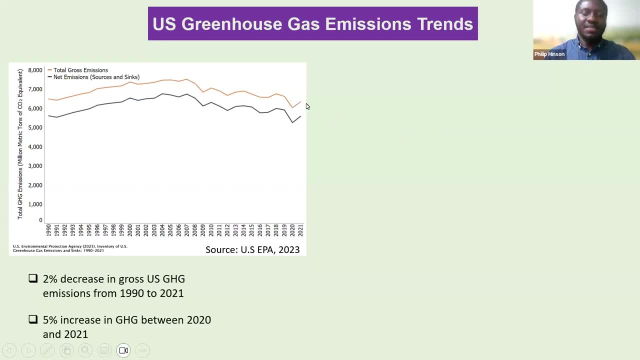 So the rate of growth- the rate of growth in 2020- has decreased by about 2%. So the rate of growth has increased by about 2%. So the rate of growth has decreased by about 2%. This clearly indicates that there's a strong relationship. 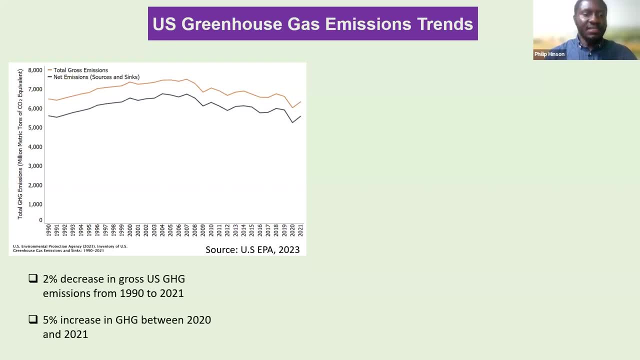 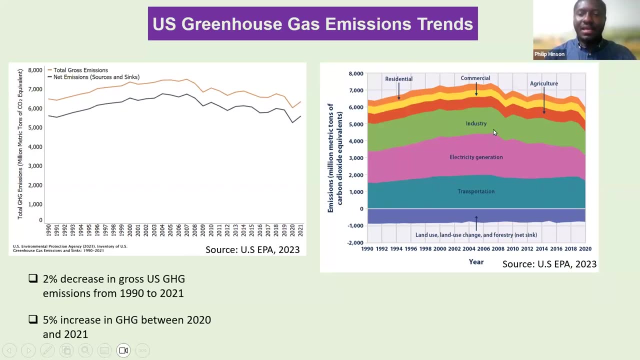 between human activity and greenhouse gas emissions. Electricity generation, transportation and industry sectors are the three primary sources of greenhouse gas emissions over the years, And these sources account for 70 to 75% of greenhouse gas emissions. The only sector that acts as a sink, or a net sink for greenhouse gas emission. 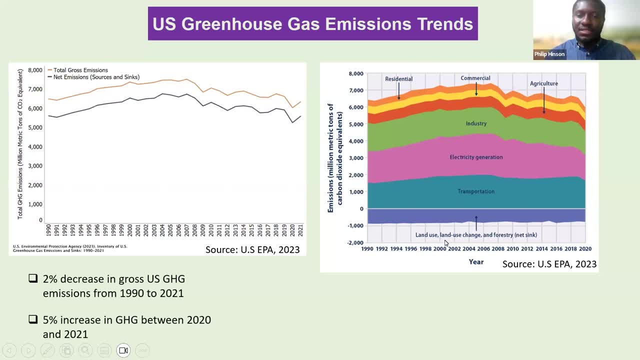 is land use in the forestry sector. So since 1990, the forestry sector has acted as a net sink, which means that that sector absorbs more carbon dioxide from the atmosphere or removes more carbon dioxide from the atmosphere than it emits. So in 2021, the land use and forestry sector 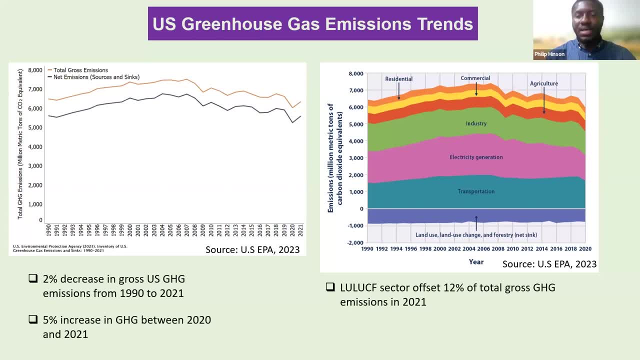 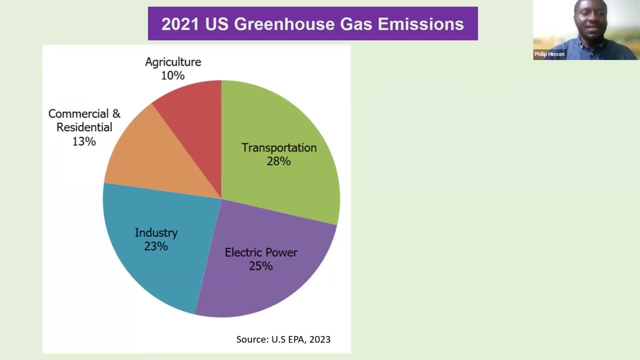 offset about 12% of the total gross greenhouse gas emissions in the US. Agriculture contributes about 10% to the total greenhouse gas emission in 2021. This number is a drop from 2020, which was about 11.4%. 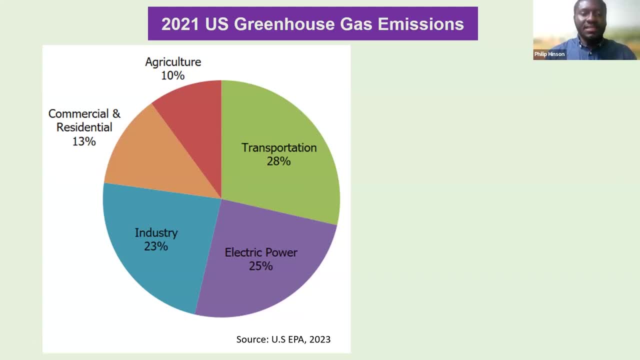 So now USDA has invested a lot of money into climate smart projects to investigate ways to reduce greenhouse gas emissions as a result of, or from, agriculture practices. The major agriculture practices, or some of the agriculture practices that lead to an increase in greenhouse gas emissions, include livestock. 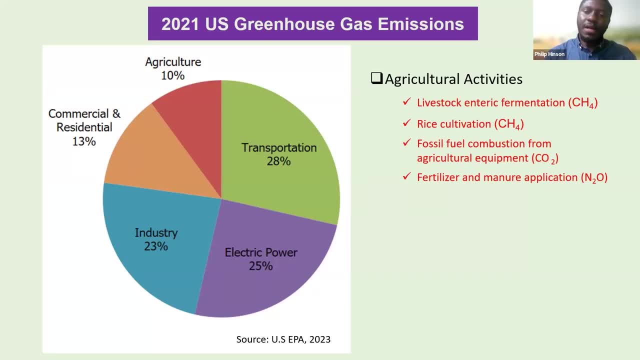 and teric fermentation, And this is the process whereby a micro or a microorganism in the rumen of ruminants breaks down carbohydrates into simpler form. So, during the process of breaking down carbohydrates into simpler form in the rumen of ruminants, 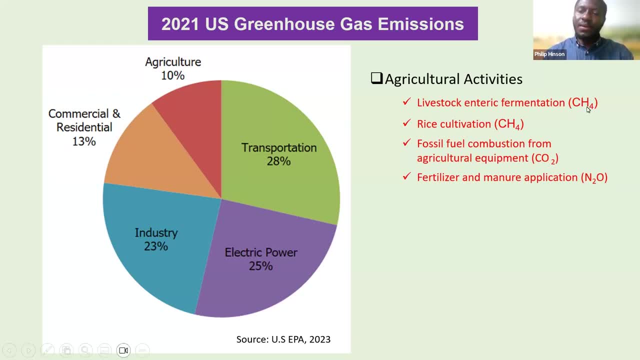 they produce lots of methane, or methane is a byproduct of that natural process. So livestock and teric fermentation is a major source of methane production And rice cultivation is also a major source of methane production. So you know rice is grown in flooded areas. 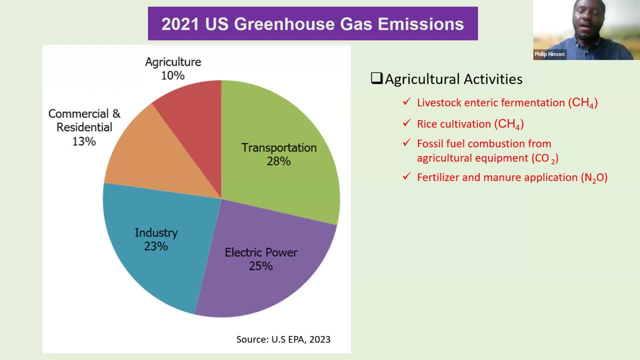 which is an ideal opportunity for anaerobic bacteria to produce methane. So the use of fossil fuel combustion from agriculture equipment also contributes to carbon dioxide emission, And fertilizer and manure application are major source of nitrous oxide emission, So agriculture is the largest source of nitrous oxide emission in 2021,. 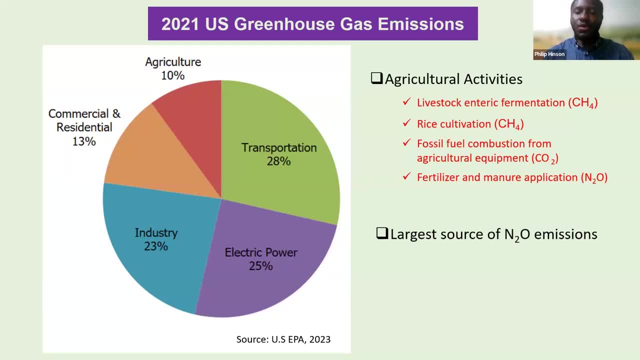 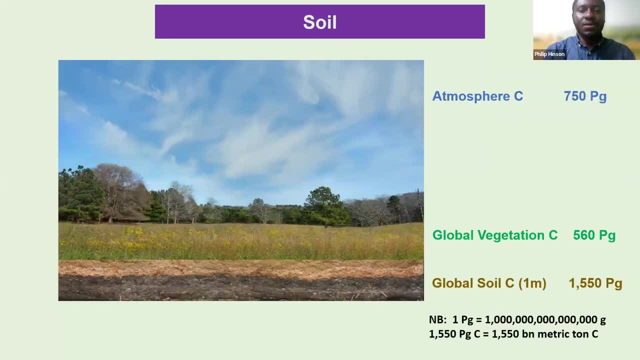 accounting for about 75% of the total nitrous oxide emission in the US. We cannot find climate change without using soil as our weapon, And the reason I say this is because soil is extremely, extremely important or it plays a critical role in the global carbon cycle. 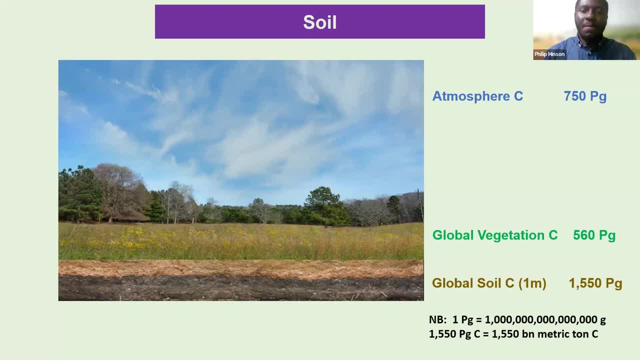 Soil has huge or massive amounts of carbon. The amount of carbon in soil is more than the amount of carbon in the atmosphere plus the amount of carbon in global vegetation. In fact, it has been estimated that if you take a meter deep soil, 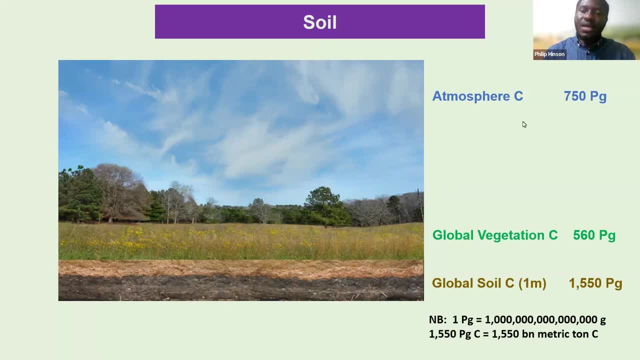 the amount of carbon in a meter deep soil is 1,550.. And this number, or this amount, 1,550 petagram. and this number is two times higher than the amount of carbon in the atmosphere And nearly three times the amount of carbon in vegetation or global vegetation. 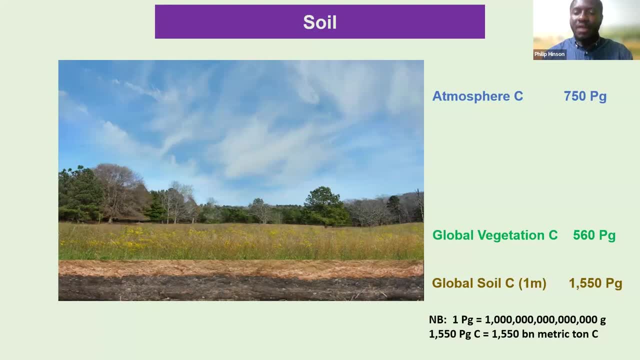 So what this tells you is: we have a lot of carbon in the atmosphere, And keep in mind that one petagram is equivalent to 10 to the power of 15 grams. So 1,550 petagram of carbon is equivalent to, or is equal to, 1,550 billion metric tons of carbon. That is a lot of carbon in the 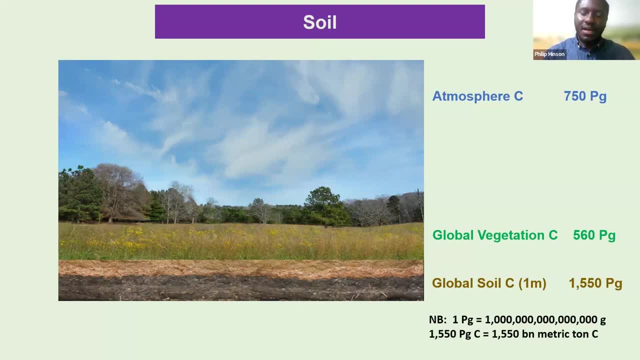 soil. So, with soil having such huge amounts of carbon, small changes in carbon in the soil can drastically or significantly affect global carbon cycle and also the concentration of carbon dioxide in the atmosphere. It is also worth mentioning that, although we know we have huge amounts of carbon in the soil, we also know that our soils have the capacities to store. 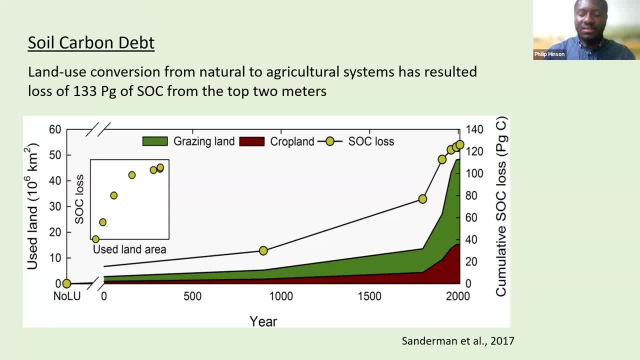 more carbon. We know this because our soils have been over-exploited since the dawn of agriculture, which was about 12,000 years ago. Jonathan Senderman in 2017, Jonathan Senderman in 2017, Jonathan Senderman in 2017,. 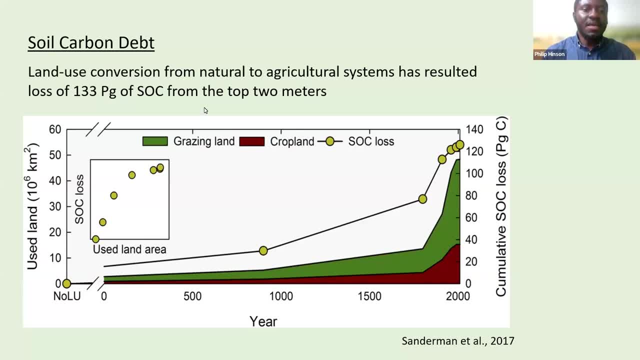 Jonathan Senderman and his colleagues in 2017, estimated that the conversion of natural systems to agricultural systems resulted in the loss of about 133 petagrams of soil organic carbon from the top two meters. So what this does is it gives us the opportunity to change the way we manage our agricultural land, using regenerative 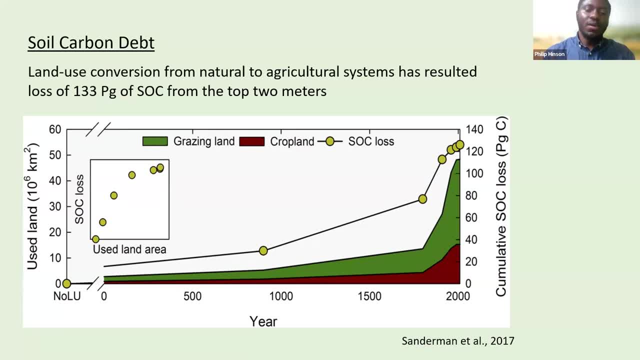 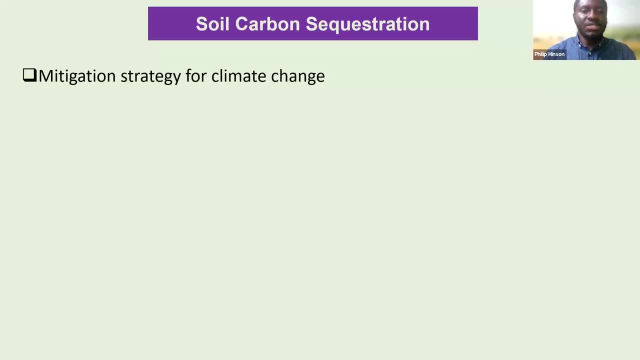 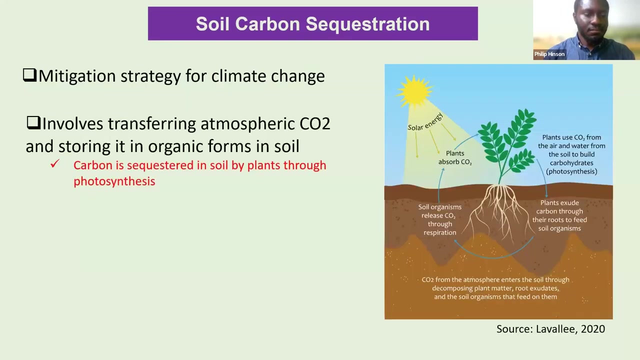 practices to put back this lost carbon into the soil. We can put back this lost carbon into the soil through a process called soil carbon sequestration, And soil carbon sequestration is a viable climate change mitigation strategy. So soil carbon sequestration simply means: 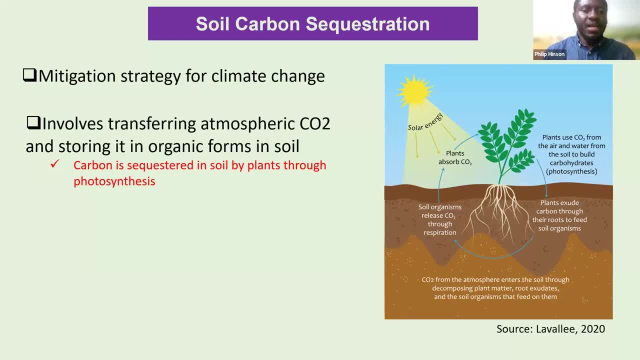 it involves plants absorbing atmospheric carbon dioxide through the process of proton synthesis and pumping this carbon dioxide into the soil. So soil carbon sequestration increases soil carbon content, and it is governed by a delicate balance between inputs, such as photosynthetic inputs via litter and roots, exudation and output. So soil carbon sequestration increases soil carbon content. 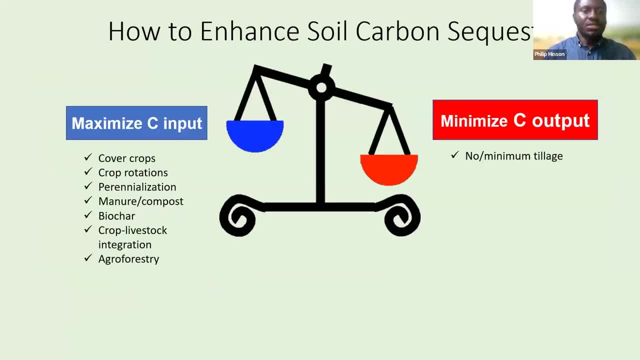 and output, such as decomposition. So to enhance soil carbon sequestration, we need to maximize carbon inputs And we can maximize carbon inputs by increasing biomass inputs into the soil. And we can minimize carbon outputs from the soil by minimizing the amount of carbon that is produced. So we can 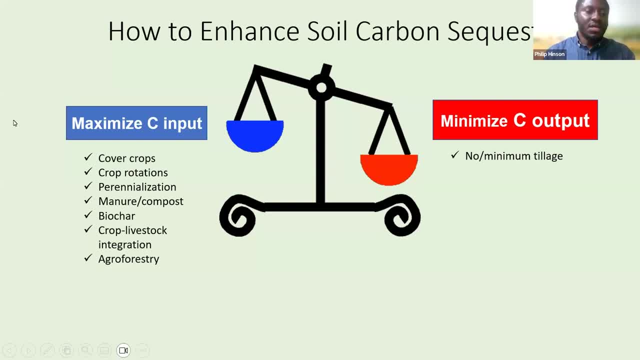 maximize carbon inputs by increasing biomass inputs into the soil. And we can minimize carbon inputs from the soil by increasing biomass inputs into the soil. And here are some of the ways we can increase biomass inputs into the soil: through cover cropping, crop rotation, adding perennials. 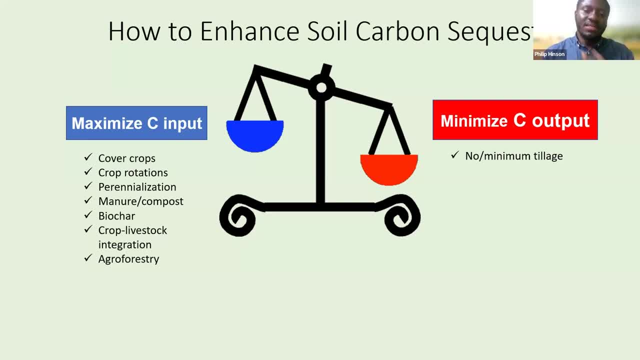 intensifying crop livestock integration And at the same time we also need to minimize soil disturbance and add more carbon elements So we can maximize carbon inputs by increasing carbon inputs bands. So if we minimize soil disturbance we reduce the oxidation of carbon from the soil. 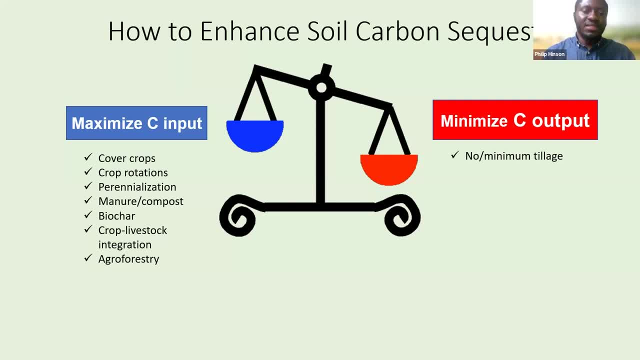 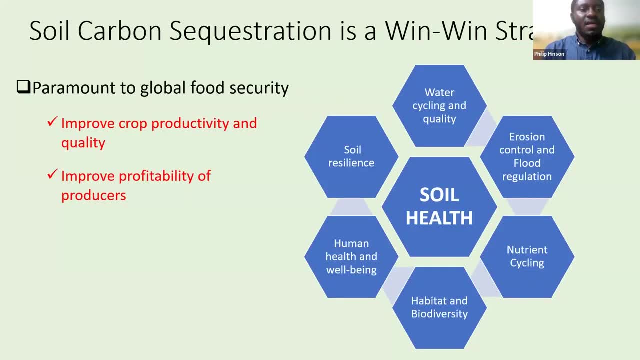 So you have to make sure your input is much, much greater than your output for you to sequester carbon. We know that increasing soil carbon is critical to fighting climate change, but not only that. it is also important to global food security, now and in the future. An increase in soil carbon. 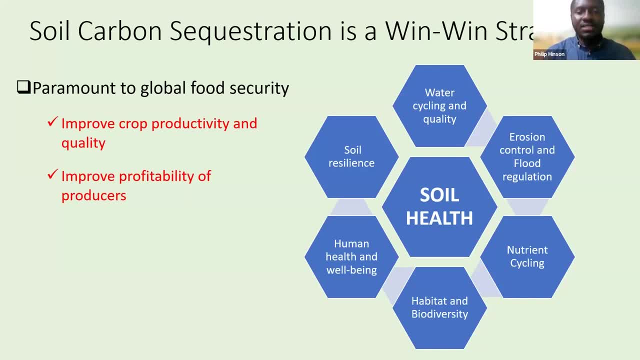 improves crop productivity and quality, and it also improves the profitability of producers. So an increase in carbon, which is also improving soil health, has so many other benefits or co-benefits, such as water cycling and quality. So water filtration and purification, improving erosion control and frat. 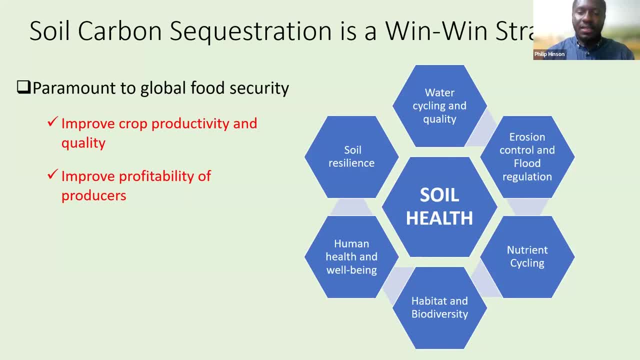 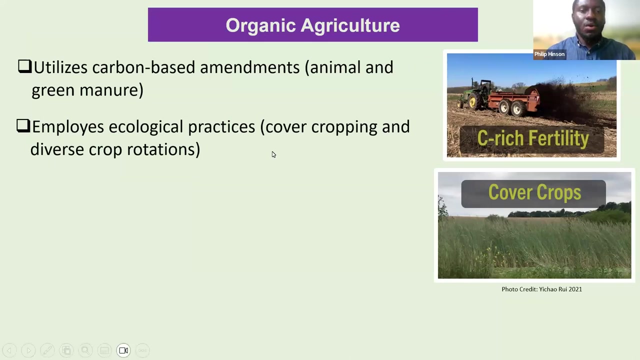 regulation, nutrient cycling, habitat and biodiversity, and many, many more. So soil carbon sequestration is essentially a win-win strategy for humans, for producers, for consumers and also for our environments. Now, unlike conventional farming, organic agriculture or organic farming avoids the use of. 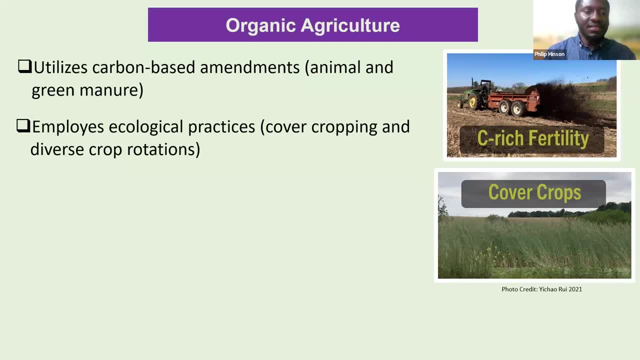 synthetic pesticides and synthetic fertilizers, but instead relies or utilizes carbon-based amendments such as animal and green manure, and also employs ecological practices such as cover cropping and diverse crop rotation, in a holistic, organic approach to improve the performance of the system. So organic farmers tend to have longer crop rotation and more diverse. 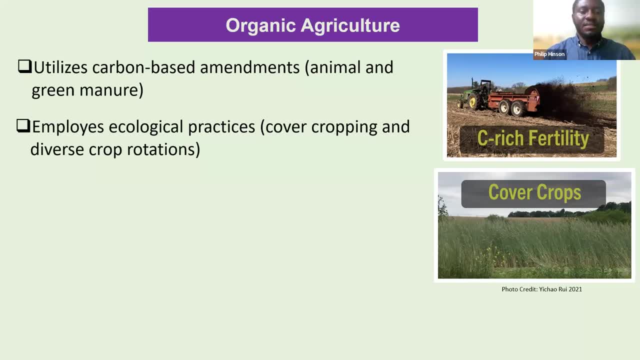 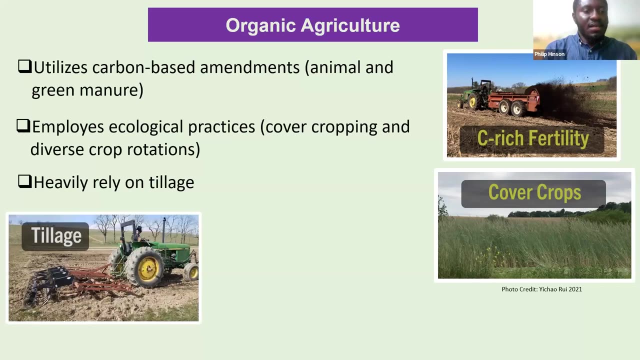 cropping systems than conventional farmers. This is because organic farmers need to utilize cover crops and crop rotations to break the reed and pest cycle, as well as to optimize nutrient cycling. But tillage is the Achilles heel of organic farming. as many, many organic farmers, 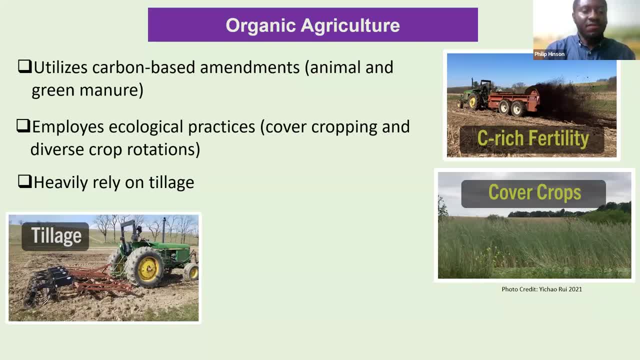 rely heavily on tillage for weed control. We know tillage or frequent use of tillage destroy soil structure and leave the soil prone to erosion, as well as negatively affect soil health and negatively affects many, many soil health parameters, including soil organic matter. 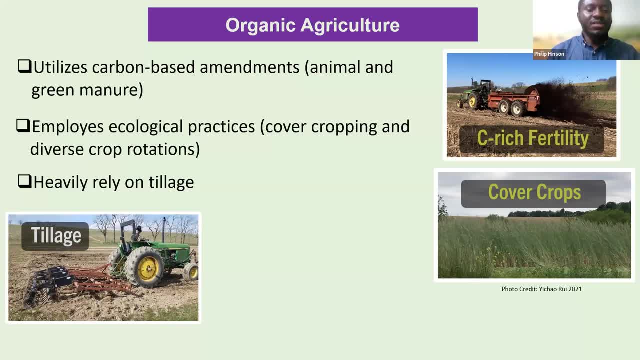 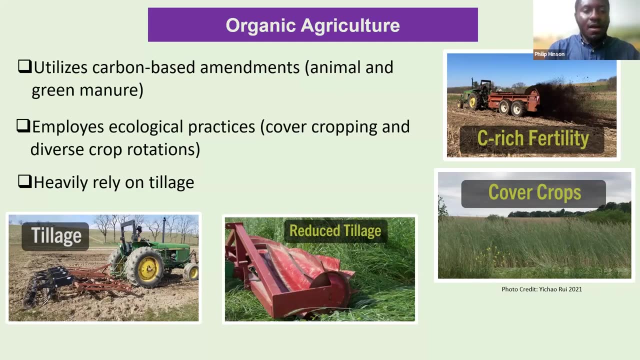 And we also know that in organic systems we cannot completely eliminate tillage at this point in time. But what we know is we can reduce tillage And here at Rodale Institute- or Rodale Institute has been at the forefront of promoting reduced tillage in. 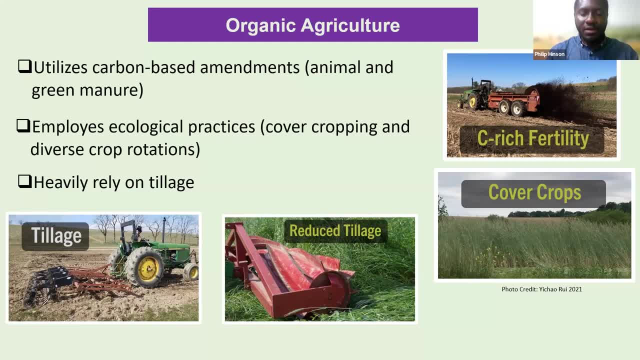 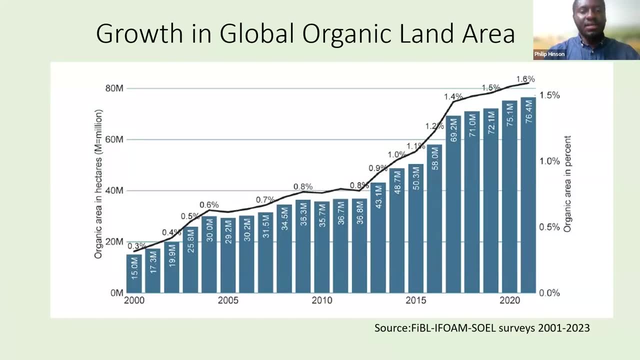 organic systems using the roller crimper. So the organic industry is rapidly growing in many fronts in a consumer demand front from the market, sorry, from the market front, the areas and organic farming. So if you look at multiple sectors within the organic industry, everything 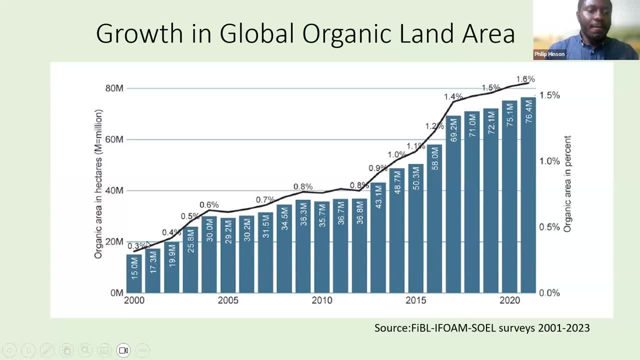 is growing. So if you look at multiple sectors within the organic industry, everything is growing. So, for example, area under organic in 2000, globally has increased by over five-fold from 50 million hectares to about 76.4 million hectares. You can see there's been significant. 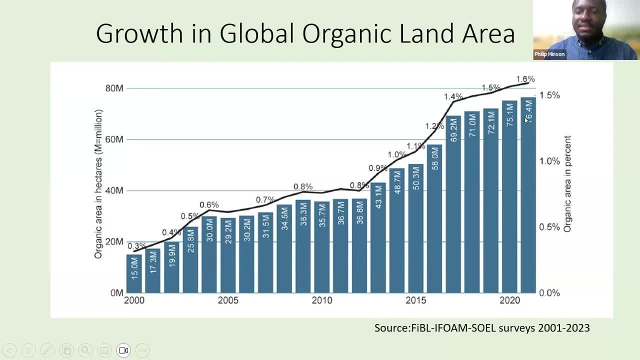 and very drastic growth, But at 76.4 million hectares this just represents only 1.4 million hectares, And this is still very small. Then the big difference is that almost every sector that grows in organic systems is just about 1.5% of the total global agricultural land area. 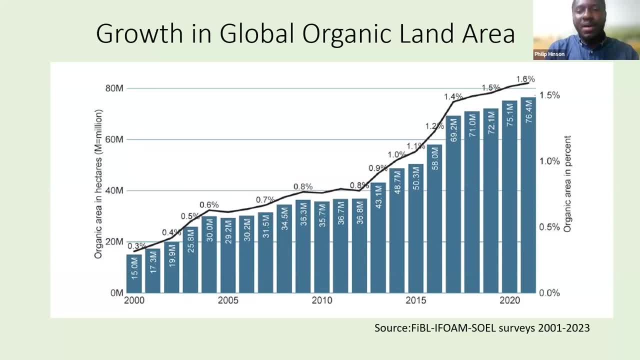 So, although we are growing, which is good, but it's still small. it's just 1.5% of the total global agriculture area, And this number in the US is much lower. In the US, the area under organic is about 3.2 million hectares, And it's less than 2.3 million hectares in terms of total agricultural land. in the US, In terms of total agricultural land, it's about 0.5 million hectares and it's much, much. lower In terms of total agricultural land. it's about 2.3 million hectares and it's much, much lower. If we take every sector under organic, we can see the growth over the course of the 18 years, which is a significant 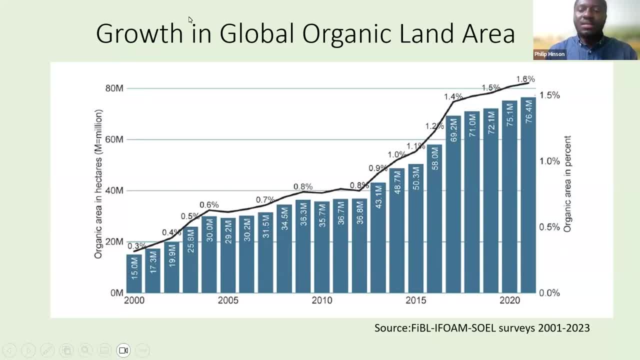 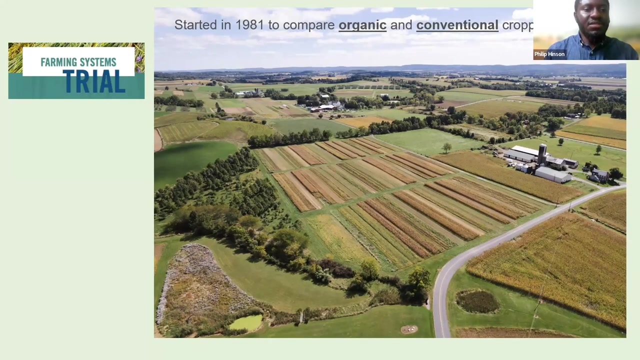 And it represents only 0.6% of the total agricultural land in the country. So this calls for the need for improvements, like we need more areas under organic farming. Riddell Institute has the Farming Systems Trial, which is a long-term experiment which was started in 1981.. 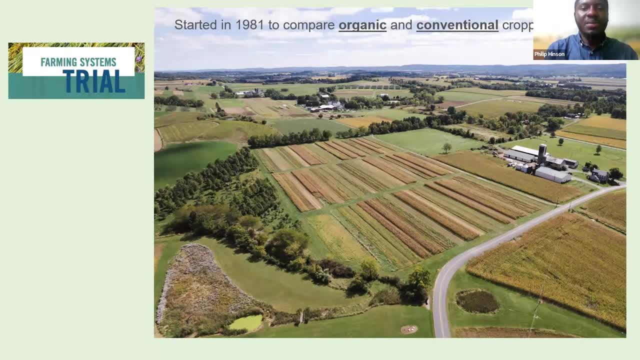 To compare organic and conventional cropping systems. So with the Farming Systems Trial still running, it is the longest side-by-side comparison of organic and conventional green cropping systems in North America. The Farming Systems Trial has contributed immensely to the organic industry in the United States. 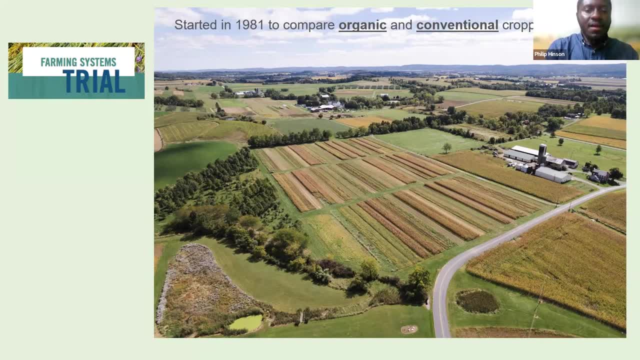 For example, if you are familiar with the Organic Food Production Act, that act was enacted in 1990, that was nine years after the Farming Systems Trial was established- And the Farming Systems Trial contributed immensely in developing that act. The Farming Systems Trial sits on a six-hectare farmland located in Coast Town, Pennsylvania. 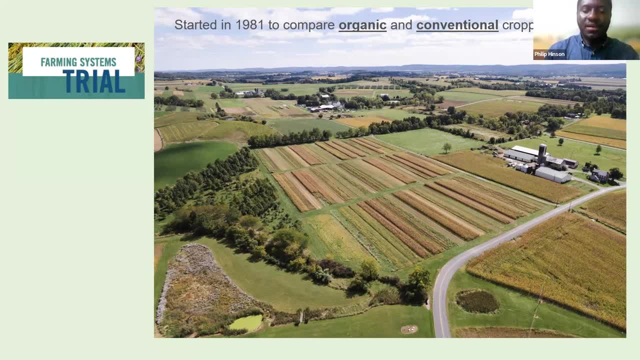 which is where the main campus of Riddell Institute is. So Coast Town, Pennsylvania, is about two-hour drive west of New York City and about one-hour drive north of Philly. So in 2021, we released our 40-year report, or the 40-year report for the Farming Systems Trial. 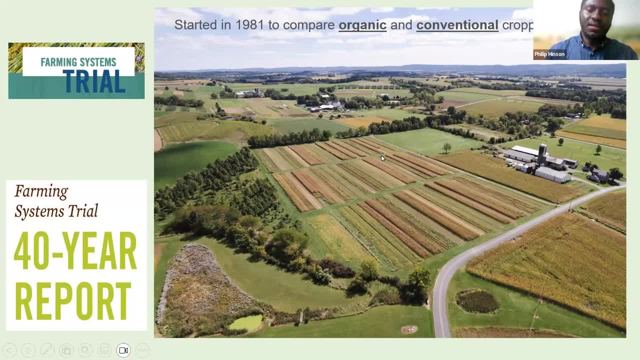 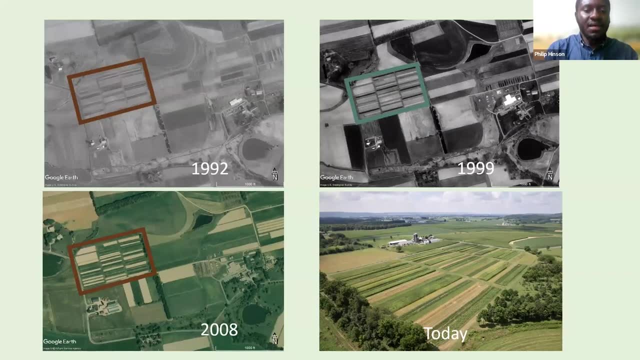 And the image you can see, you are seeing on the screen, is the Farming Systems Trial. So here are some other examples. There are some other area images of the Farming Systems Trial over the years. So Farming Systems Trial in 1992, Farming Systems Trial in 1999, and Farming Systems Trial in 2000,. 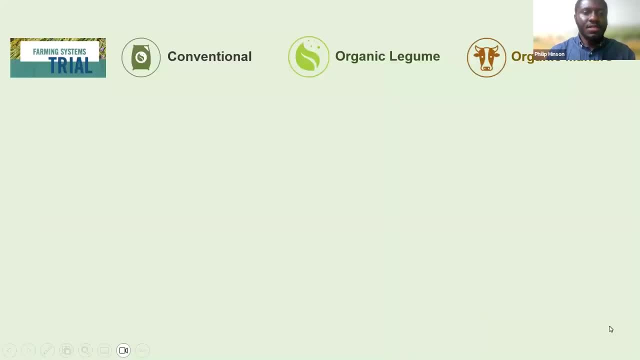 and finally Farming Systems Trial today. So in the Farming Systems Trial there are three cropping systems- conventional, organic legume and organic manure- And these systems vary In cash. crops cover crops and imports. So the conventional system follows a three-year rotation, which is corn, corn, soybean. 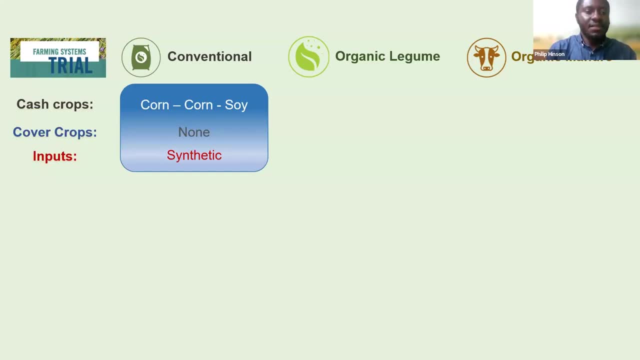 There's no quark crop in that system. So this simple rotation is practiced by most or many producers in the Mid-Atlantic region, And we are using corn and soybean because they are the two major grains produced in the US- The total cropland under grains in the US is about 100 million hectares- and corn. 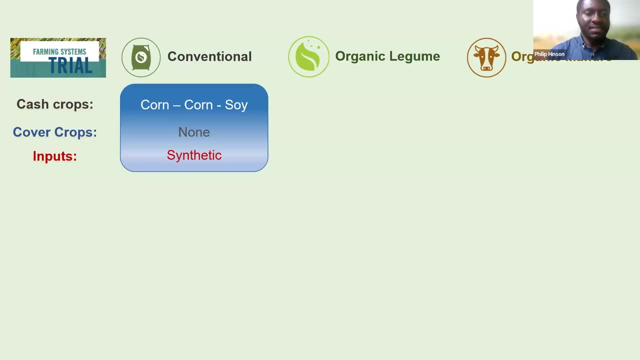 and soybean is produced in about 70 million hectares of that, So almost 70% is under corn and soybean. So you can't have a conventional system without having corn and soybean in it, which are the two major cash crops. There are no cover crops in the system, like I said. 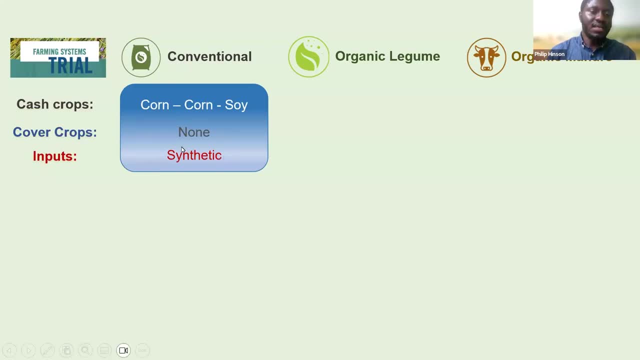 and this system heavily relies on synthetic inputs, synthetic pesticides and synthetic fertilizer. Then we have the organic legume system, which follows a four-year rotation of corn, oats, soybean wheat, And in this system we have cover crops, rye and hairy veg. 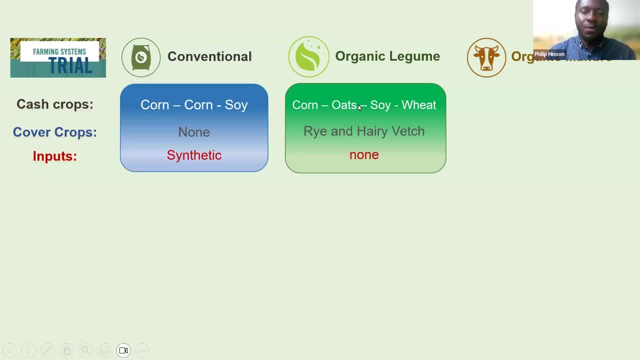 I must say that during the oats phase we interseed with clover And in this system there's no input, So we rely solely on biological nitrogen fission from the legumes. So you know that our Earth's atmosphere has about 78% of nitrogen. 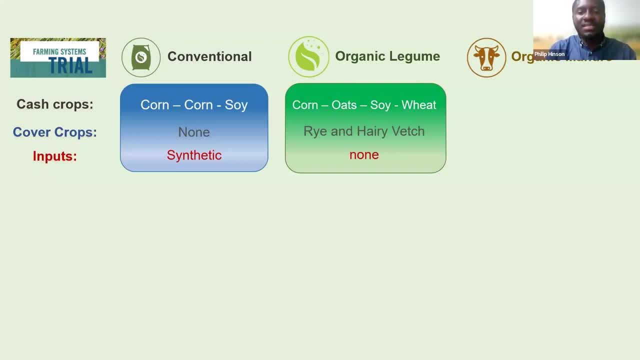 but most plants cannot utilize the amount of nitrogen we have in the atmosphere, except only few or specialized plants like legumes. So legumes are able to form a symbiotic relationship with rhizobia or bacteria in the soil to break down the strong nitrogen bond and make nitrogen available for plants use. So we solely rely. 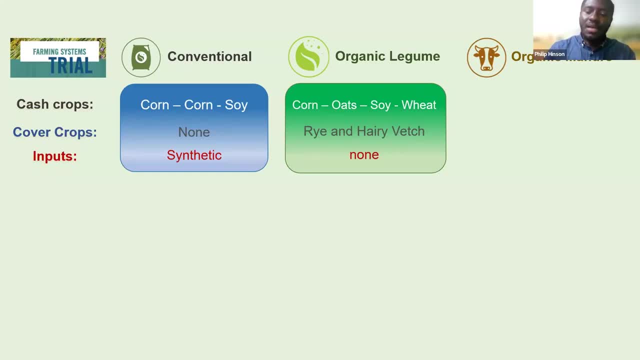 on biological nitrogen fission in the organic legume system. The manure system is much, much longer and diverse. So on top of the four-year rotation in the legume system, we have a three-year hay phase and a corn silage phase, as well as wheat. 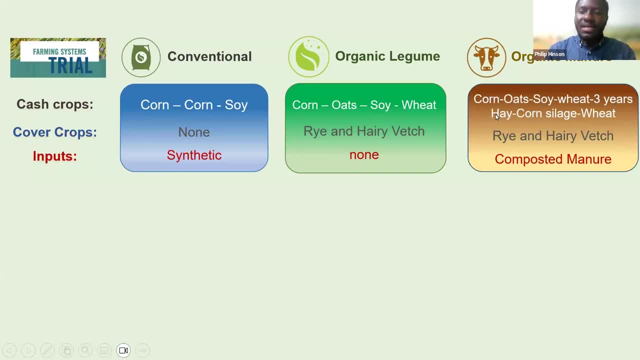 So the manure system is a nine-year rotation. The three-year hay phase consists of alfalfa and orchard grass And we have rye and hairy veg as our cover crop in this system And we apply composted manure in this system. 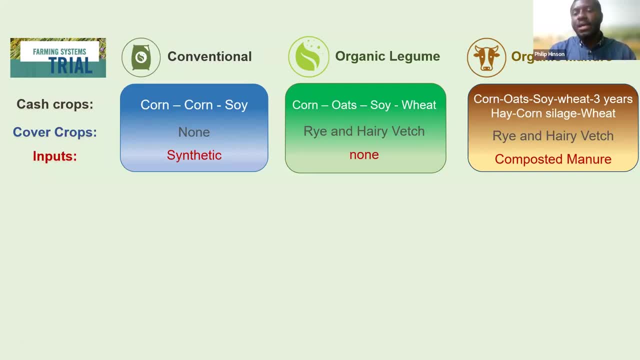 So during the nine-year phase, we apply composted manure during the oats phase of the rotation and during the corn silage phase of the rotation. So during the nine-year phase we apply composted manure only two times, at rates of about 10 to 15 tons per hectare per acre. 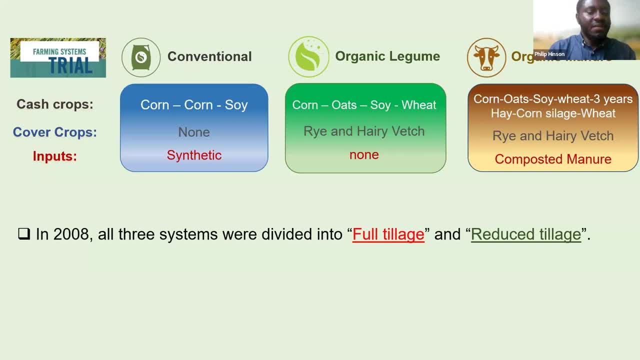 So, as I said or mentioned in the previous slide, the farming systems trial was established in 1981. And in 2000.. And in 2008, a major modification happened. So prior to 2008,, the farming systems trial was under intensive silage. 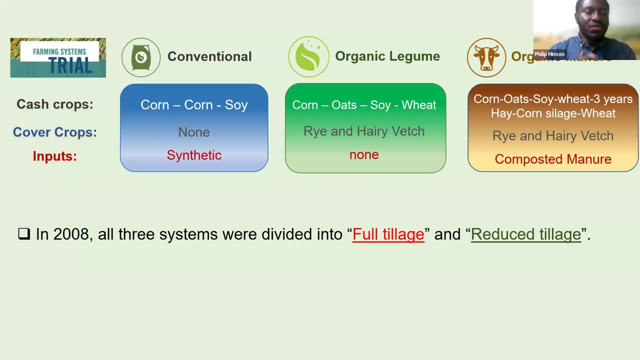 All plots were under intensive silage. So in 2008, the modification that happened was the three systems were divided into full silage and reduced silage. So we introduced a silage treatment. So we introduced a silage treatment in 2008.. 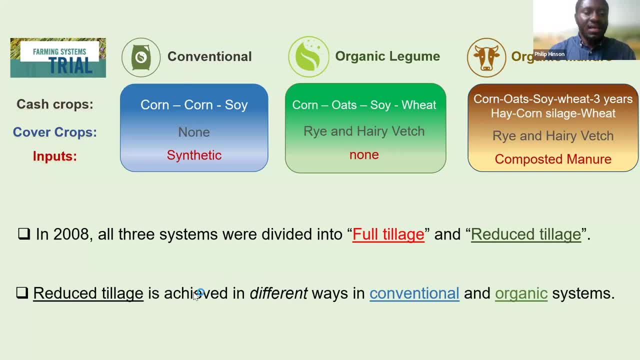 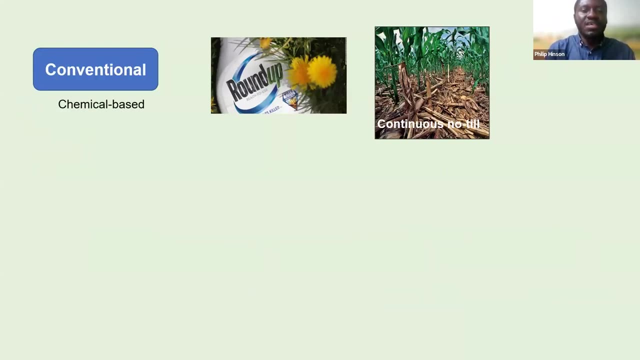 But we know reduced silage is achieved in a different ways in conventional and organic system, Because in conventional system you can use chemical-based herbicides and GMO seeds to achieve reduced silage, But in organic system we don't have that tool. 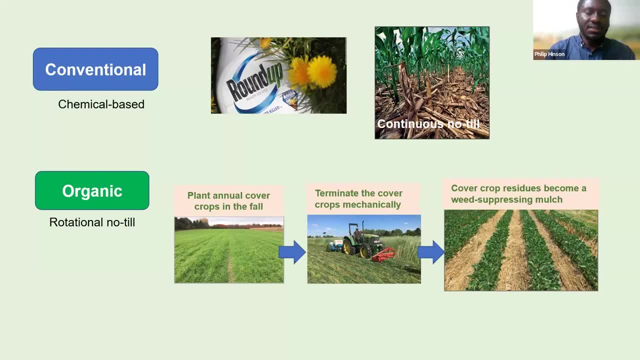 So we do what is called rotational no-till or cover crop-based rotational no-till. So what that means is we will use silage to establish our cover crop sometime in the fall, Then simultaneously terminates the cover crop mechanically using the roller crimper and also plants our cash crop into the mulch simultaneously. 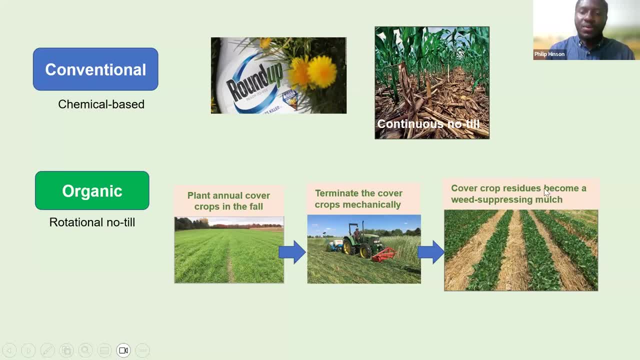 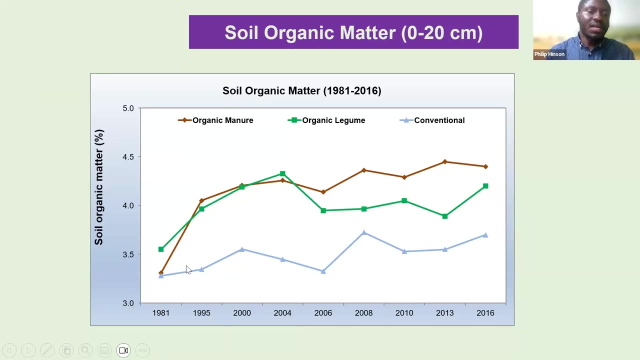 So this is the result. So you can see here, cover crop residue become a re-suppressing mulch And you can see. so this cover crop is right And you can see your silage bin. So to get into some results, when FST started in 1981, the soil organic matter levels were relatively similar. 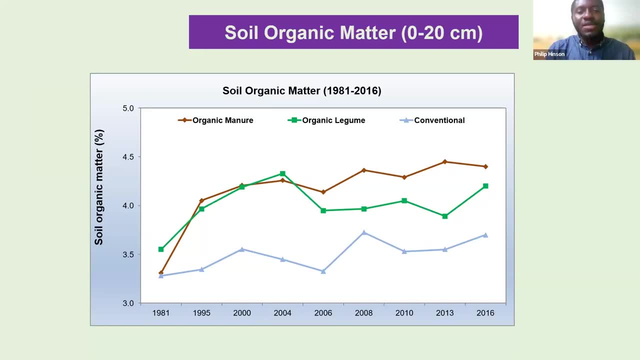 So soil organic matter can be used as a proxy for soil organic carbon or soil carbon, Because soil organic matter contains 58% carbon. So you can see here, You can see that in 1981, the three systems had relatively similar soil organic matter. 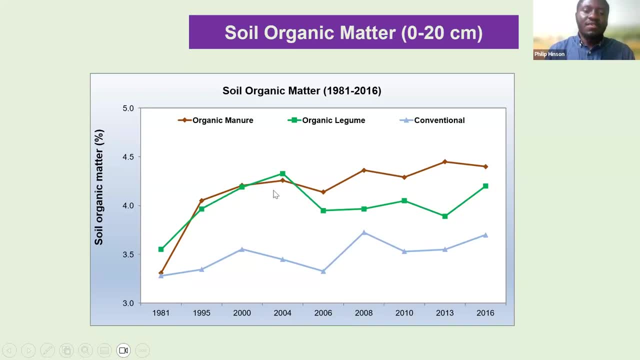 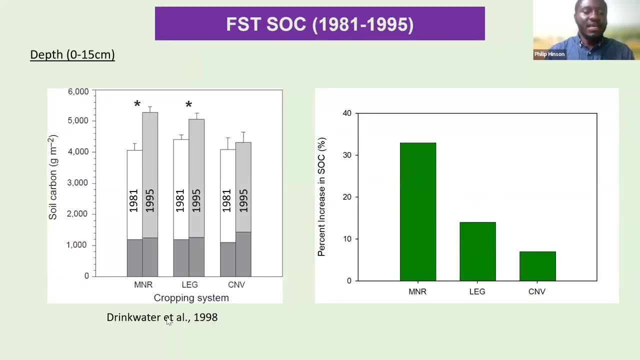 But the two organic systems increased rapidly in soil organic matter. So in 1998, Drinkwater et al published a paper on FST soil organic carbon stock From 1981 to 1995, and they found that the percent increase in the manure system from 1981 to 1995 was about 30%. 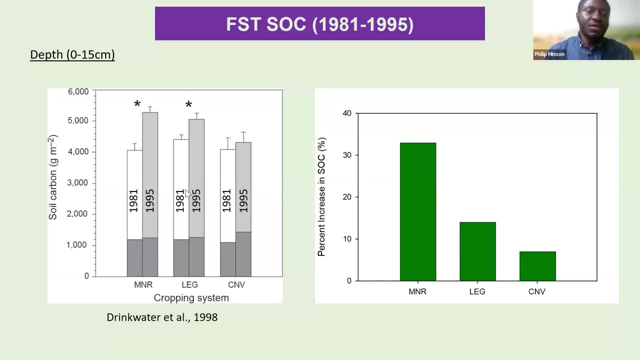 And the percent increase in the legume system from 1981 to 1995 was about 14% And it was significant. But the percent increase in the, The conventional system was only 7%. So this kind of gives you an idea on or about this soil organic carbon sequestration potential of organic farming. 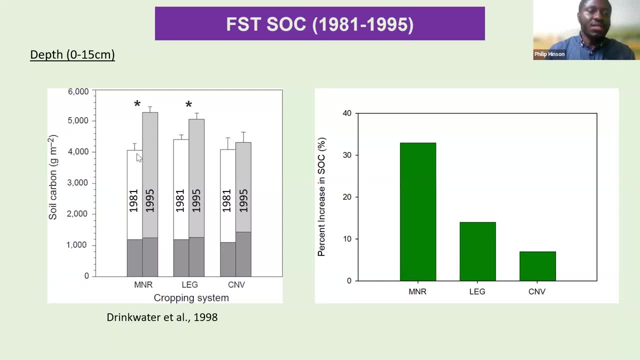 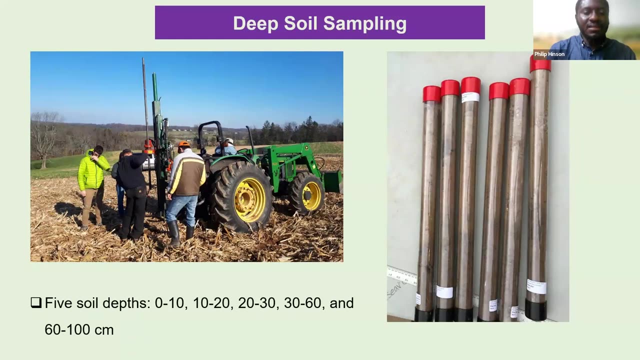 So the primary reason for the increase was as a result of crop diversification, like diversified cropping systems and cover cropping. So in 2021, we wanted to Accurately estimate soil organic carbon stock in an entire one meter soil profile. So we know that deep sampling is essential when you want to accurately estimate soil organic carbon. 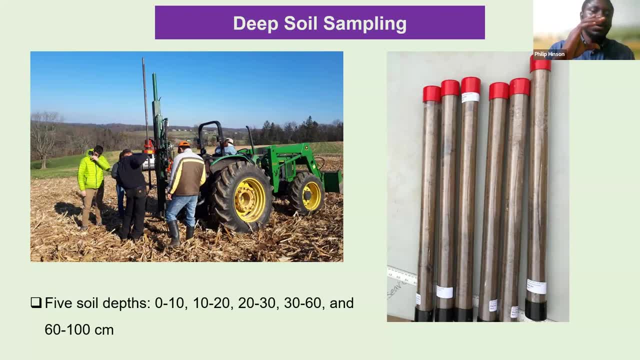 Because if you just consider the top soil, you might underestimate or overestimate your soil organic carbon And therefore you might underestimate Your soil Carbon sequestration potential. So in 2021.. We collected a meter deep soil And we sliced it into five depths. 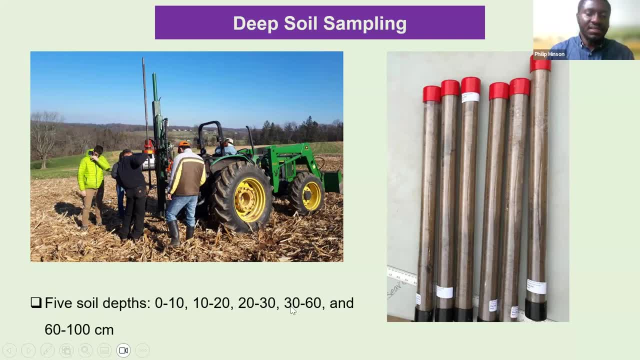 Zero to 10,, 10 to 20,, 20 to 30,, 30 to 60 and 60 to 100 centimeters, And we measured soil organic carbon For each depth As well as the cumulative soil organic carbon for the entire profile. 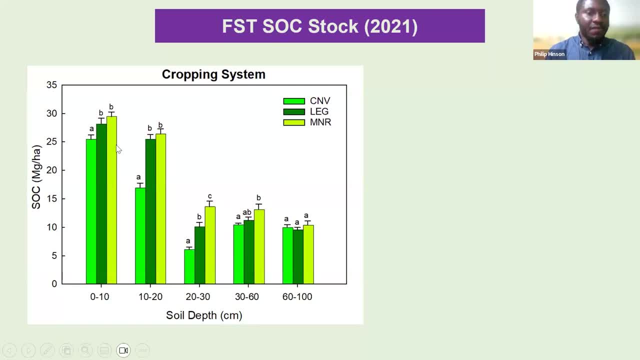 One meter profile And We found out The two Organic systems Are significantly more So organic carbon stock, That's the depth of zero to 10.. Done the conventional system And even if, if you consider 10 to 20 at this depth, 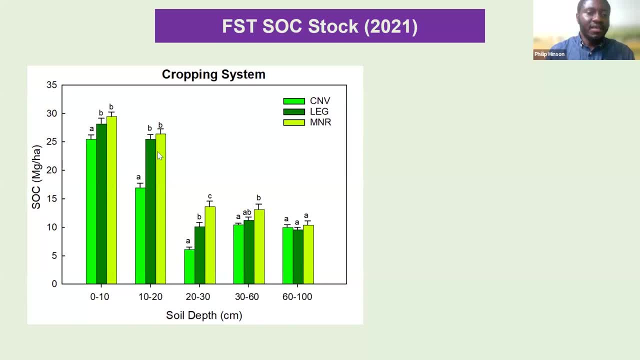 The difference is much, much greater Then: 20 to 30, the two organic systems Outperforming the conventional system, And even That's a depth as Deep as 30 to 60.. The manual system significantly had. 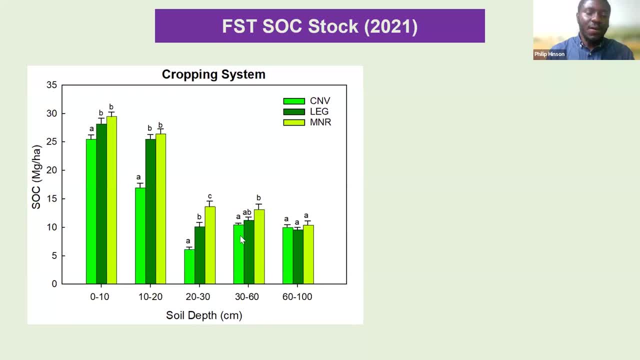 Higher soil organic carbon stock than the conventional system And, when it comes to climate change Soil Or carbon in the subsoil, Very important because those Carbon in the subsoil are not susceptible to losses, Unlike soil In a top soil. 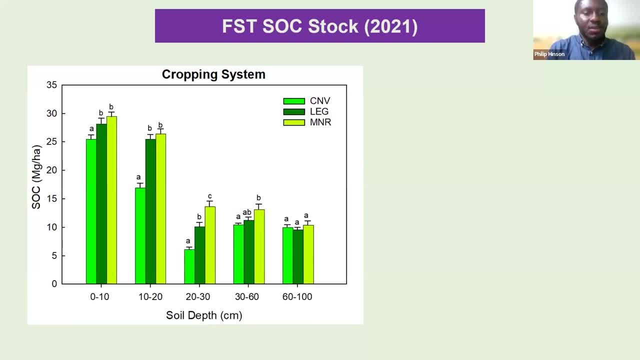 Because your top soils Will be susceptible to losses as a result of Mineralization By microbes, Rushing and many other things. So the soil, or carbon in the subsoil, Is very, very important For long-term carbon Sequestration. And Stabilization, So From Zero to 30.. We found that soil Organic carbon stock was almost 40% higher In a two organic systems than the conventional system, And From the depth 30 to 60 centimeters. 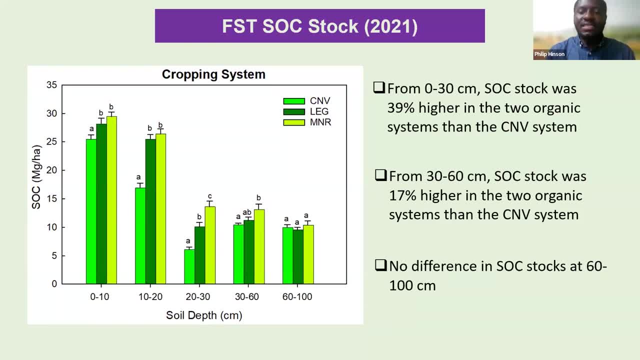 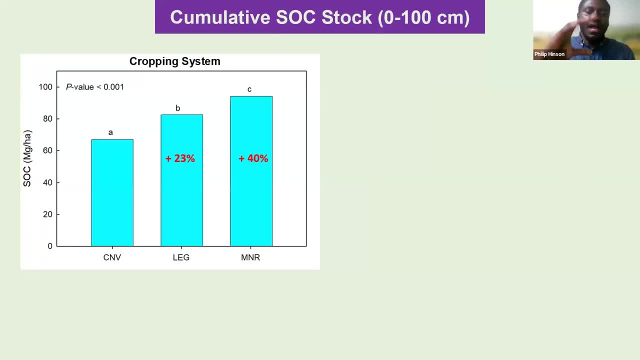 We found that soil organic carbon was 17% higher In the two organic systems than the conventional system. So when We aggregated The Entire soil sample from zero to hundred, What we are seeing is So organic carbon stock in the legume system. 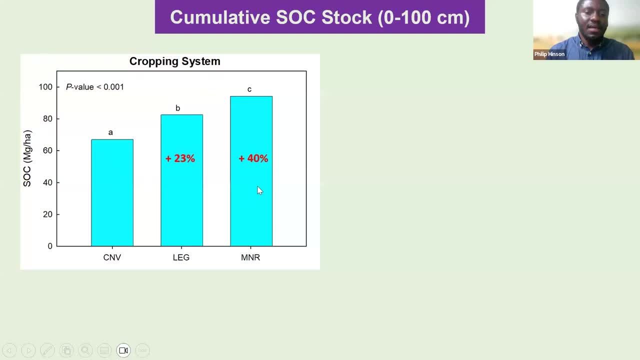 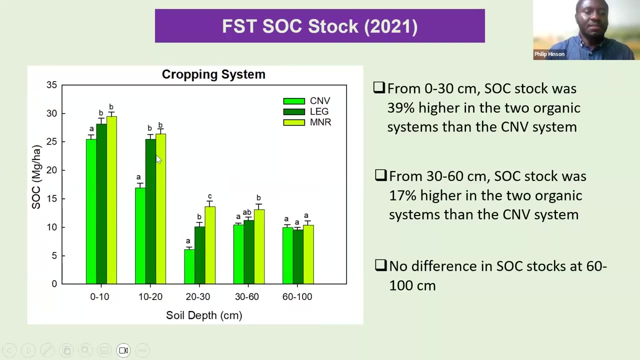 Was 23% higher than the conventional system And the manual system was 40% higher than the conventional system, And the reason We are seeing higher So organic carbon stock In the top soil Is because Of long-term ecological practices. 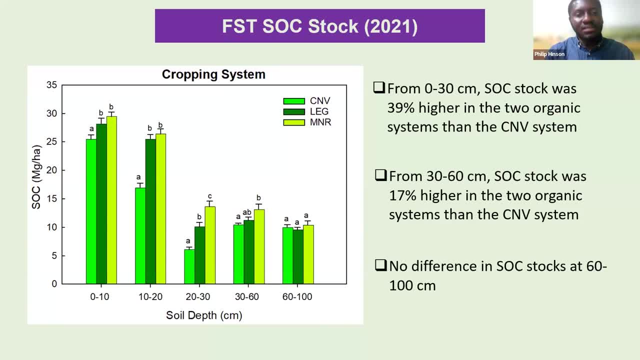 In the organic system, such as Propotations, Cover cropping And All Compost addition. What is Most striking about this graph, Particularly, is the fact that in the manual system, remember, In the legume system, remember, there was no carbon inputs. 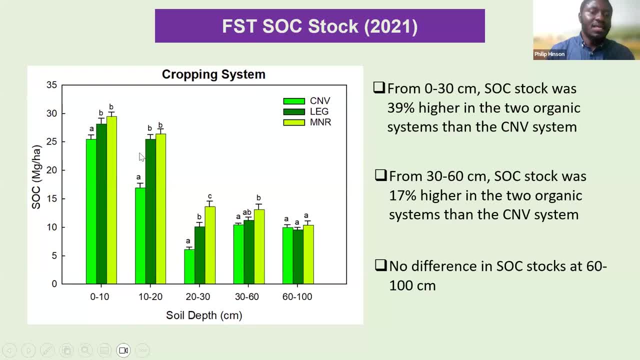 We don't add compost or manure in that system, Yet In the organic system It is. It is able to outproduce the conventional system, And the primary reason for that is Diversified cropping system And Propotation in. 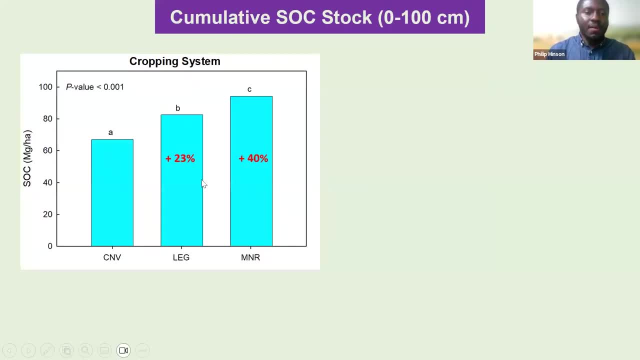 That's legume system. So The Primary reason For this increase In so organic carbon From Zero to hundred Is as a result of long-term ecological practices such as Cover cropping, Propotations And manure. 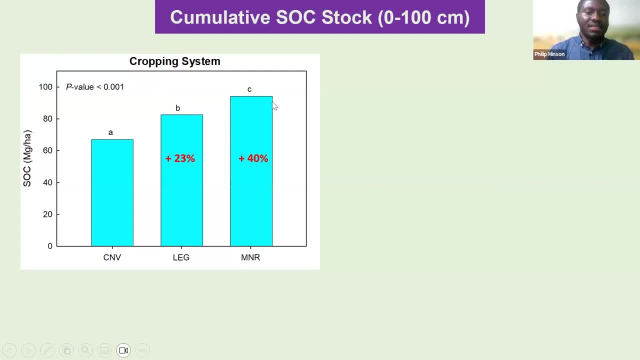 Inputs In the organic systems. Now, Surprisingly, We didn't see the effects of tillage On So organic carbon stock. So, as you can see, Full tillage, Also organic carbon stock, was about 80. Mega gram per hectare. 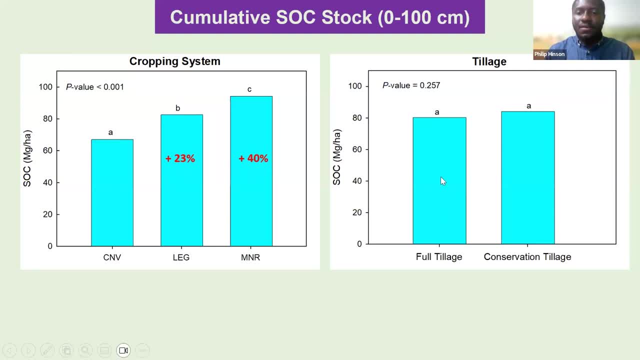 And that's conservation. tillage- Almost the same, And the reason: We didn't see the effects Of tillage On Soil: Carbon Stock, Soil, Carbon Soil, Carbon Soil, Carbon Stock. We didn't see the effects. 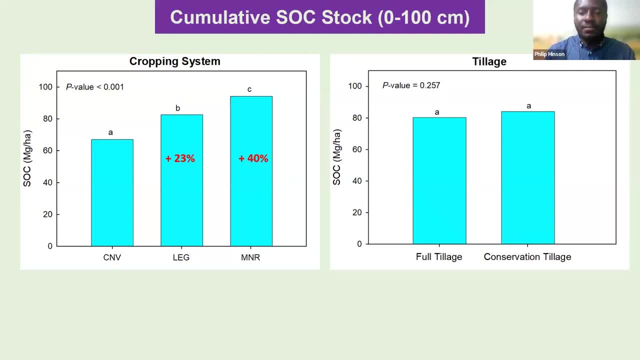 Of tillage On So organic carbon stock Where Topography And high Baseline So organic Carbon stock. So We know That We tend to lose soil As a result of Erosion And 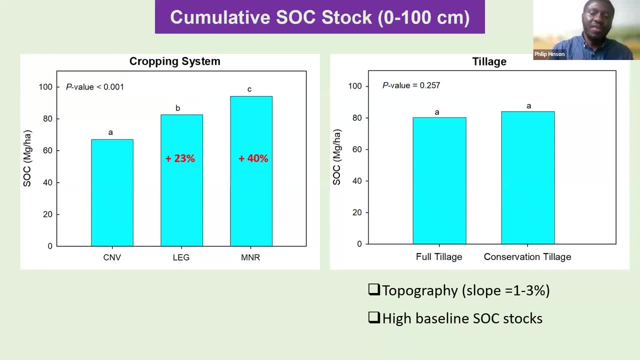 With FST Or the farming systems. Try out. The slope of FST Is relatively flat, Like one To 3%, So We don't lose Carbon As a result of Water Erosion And where. 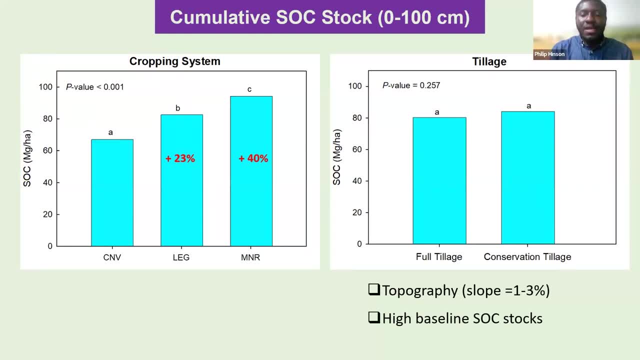 FST. Yeah, We don't lose Carbon As a result Of water Erosion. Another major Factor That contributed To the lack Of difference In Tillage Practices Is As a result. 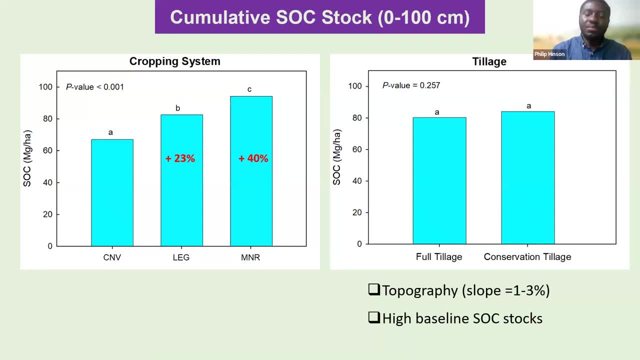 Of the high Baseline Of soil Organic Carbon Stock, So Proud To See That The Carbon Levels Were Already High In Across All Systems, As I Showed. 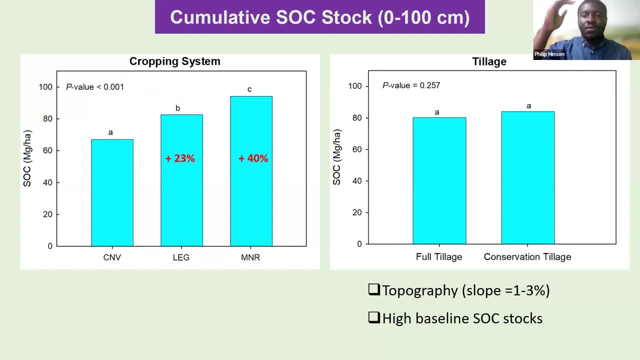 In The Soil Organic Matter Graph. The Soil Organic Carbon Levels Were Already High In Tillage System. Is A Factor Of The Climate Change And 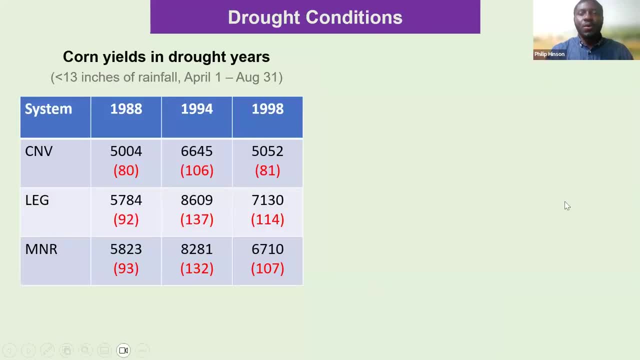 The Soil Carbon Is Very Contextual And Depends On Management And Site Specific Characteristics. So So Far Been The Different Systems In FST Perform Under. 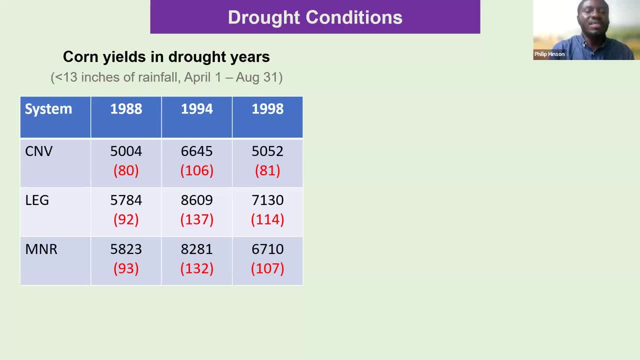 Drought Condition. So Drought Condition To Me Is A Measure Of Resilience, Like So How Resilient These Systems Are, And These Are So. 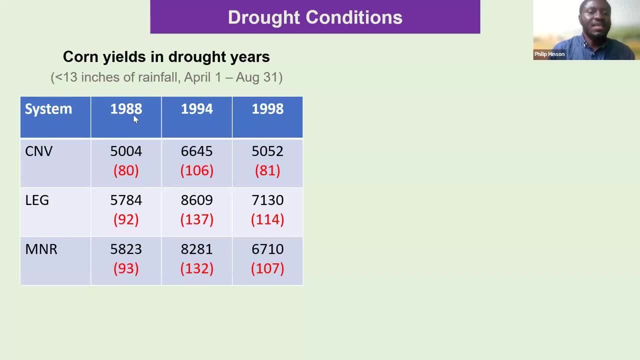 The Farming Systems Trial, We Had Moderate Drought In Nineteen, Eighty Eight, Ninety Four And Nineteen Ninety Eight. So During This 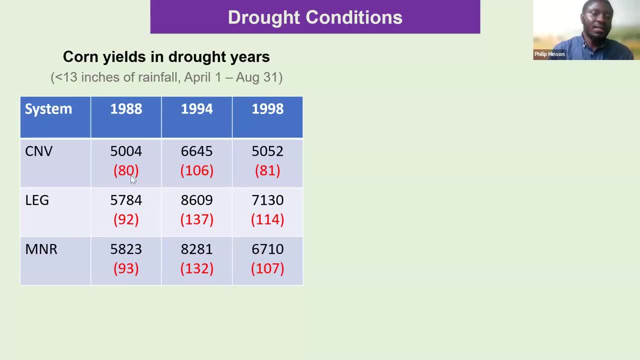 Period: Corn Yield In Nineteen, Eighty, Eight, In Ninety Four. You Can Even See A Much, Much Bigger Difference Between The Conventional System. 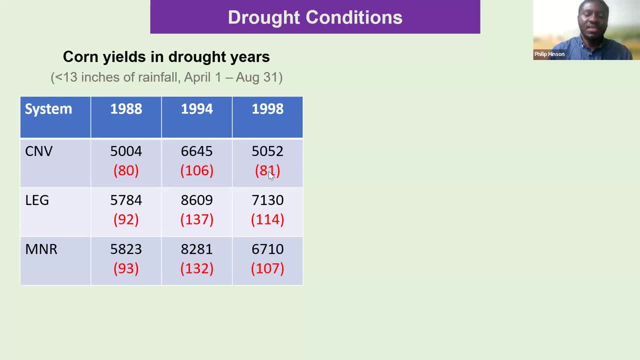 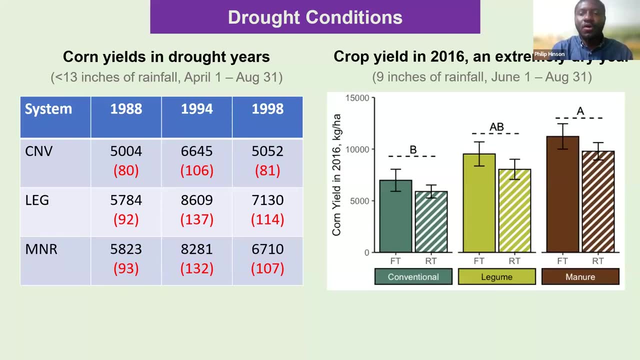 And The Two Organic Systems. In Ninety, Ninety, Eight You Can See The Legume And, Given Our Location, Does An Extremely Dry Year Because, 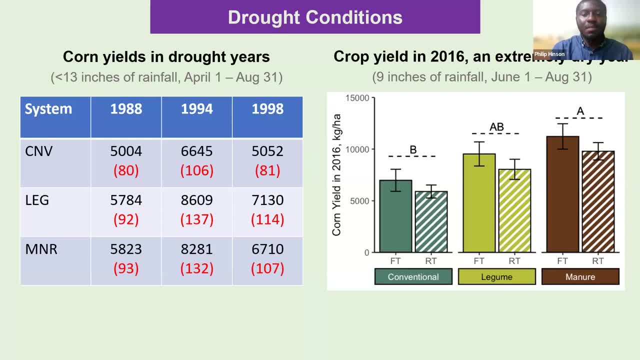 We Get About One Meter Of Rain Annually And During The Corn Production Season We Get About Twenty Nine. Two Organic Systems Outperform The Conventional. 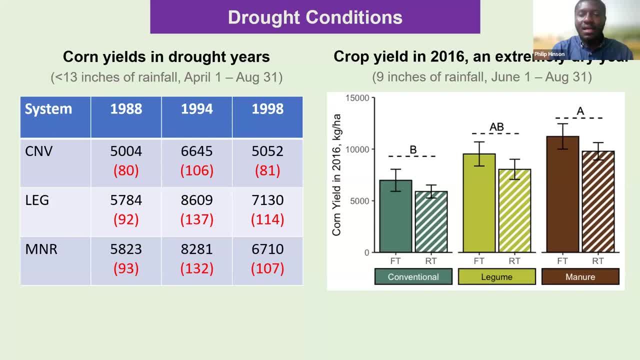 System. And Again This Shows How Resilient The Soils In The Two Organic Systems Are, So These Soils Are Able To Remain Moist. That 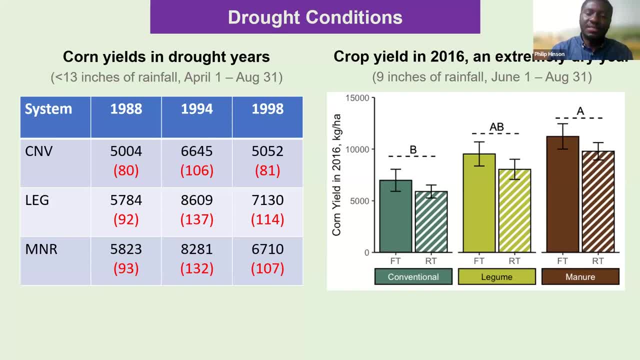 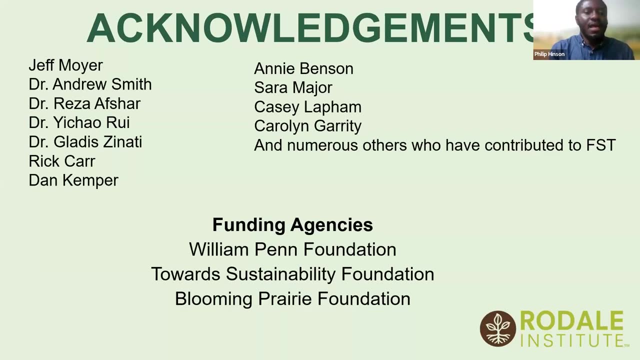 Have The Ability To Remain Moist When An Environment Is Dry And Remain Extreme. Remain Dry When The Environment Is Extremely. When The Environment Is Extremely. 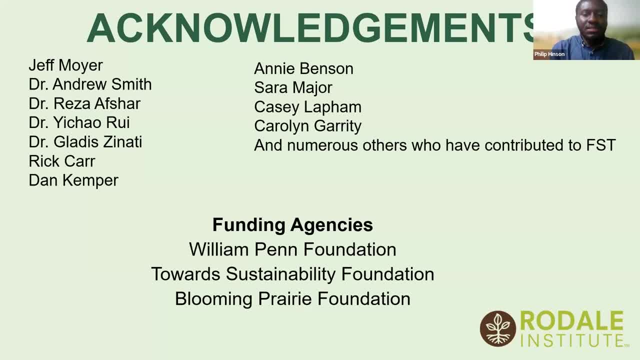 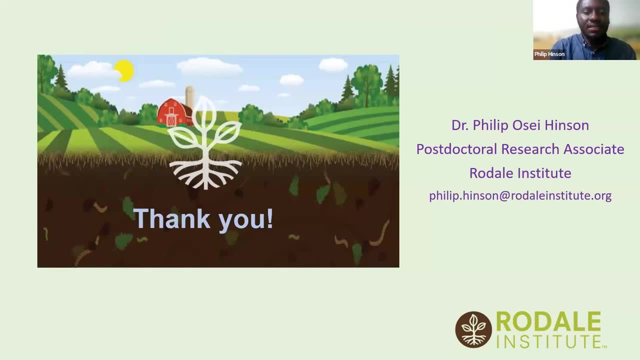 Moist. So This Is A Solution To Resilient The Soils In The Environment And This Is A Solution, And It Is A Solution To 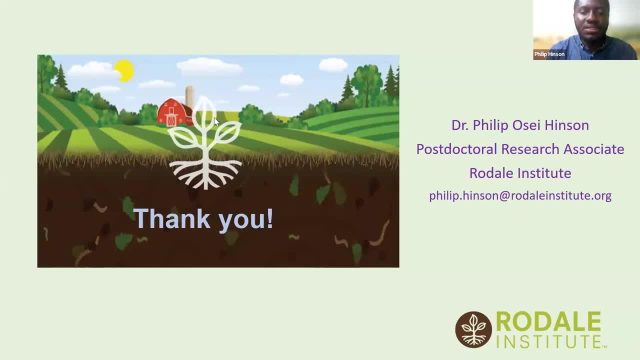 Remain And Remain And This Is A um. so the manure system tries to mimic um dairy farming, like what dairy farmers will do. so we use composted daily manure in the manual system. so if you have dairy cattle in on your farm, 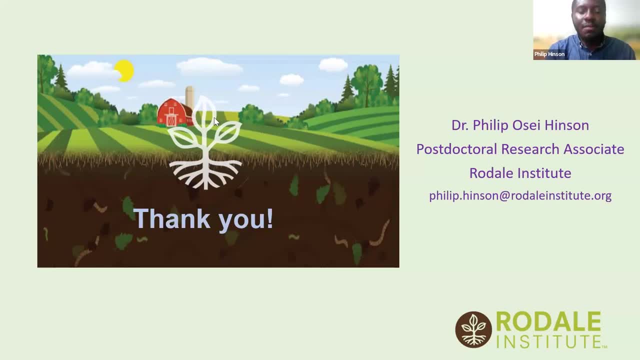 we try to mimic what's um. how does scenario pans out? yeah, so we use um composted dairy manure in the manual system. i have another question and the question is: what's the soil type of the farming systems trial? so the farming systems try. the soil type is silts, silts, loam, silts, loam soil is the. 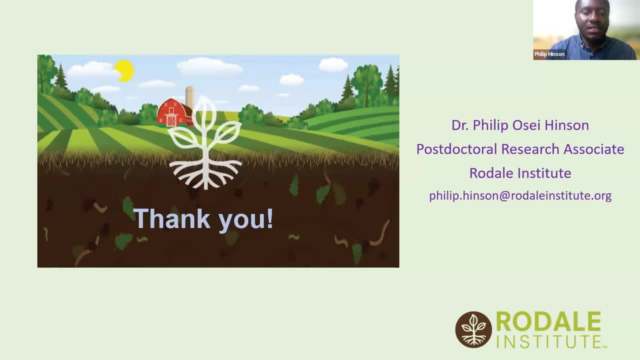 soil type of the farming system trial. and i have another question on whether we have any studies on perennials or other tree crops. we now rodeo institute. now we have a perennial scientist. she joined the team about a year ago and she is now working on perennials and tree crops. i have a question. 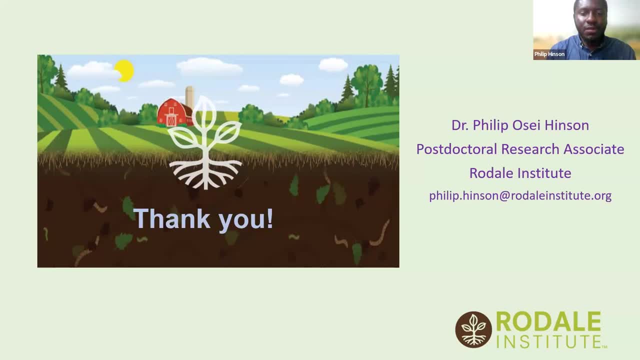 continuing conventional practices on your farm. only perpetration contributes to the program. it is time to stop, are they? we can't stop the conventional system in a farming system because it gives us an opportunity to compare the performance of the organic system to the after 40 years of the farming systems trial. we don't know. so we don't know how the system will. 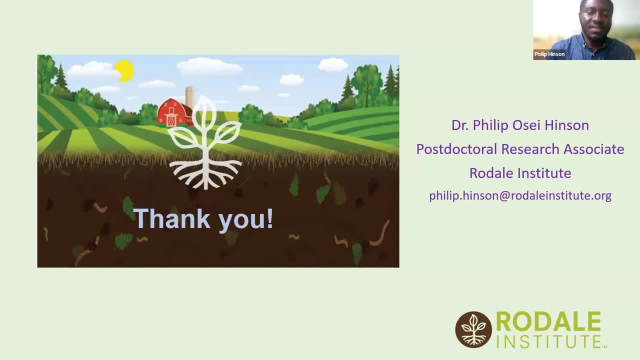 work. we still need to compare the different systems in the farming systems trial. yeah, so even after, after 40 years, we still have more like different research questions. so now we are even looking into water quality. so the effects of different um cropping systems- conventional and organic- on water quality. so 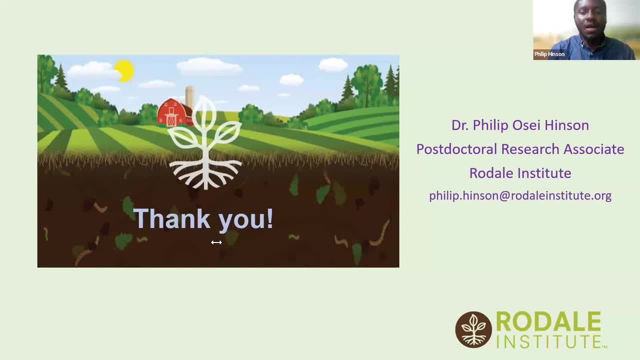 later we will see if there are still more interesting research um areas to look into we are still looking into. there are still more interesting research um areas to look into. so having the conventional systems- or having a conventional system, sorry- gives us an opportunity to have a side-by-side comparison. oh so, in 2016, slide. what do rt and ft 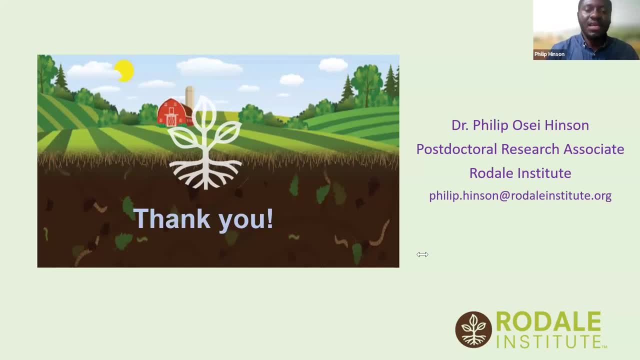 stand for. so rt stands for reduced tillage and fc stands for old leach. do you have a schedule available? orileľ does well for you. so because we have real и akhirly advantage over rt, so we may have some level of what was done and went for the legume and manure system. 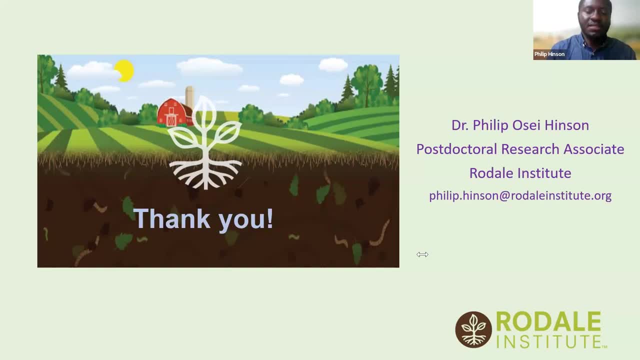 So prior to the establishment of the farming systems trial in 1981, the field was managed intensively under conventional system. So the entire five or six hectare farmland was managed intensively under conventional system. I think it was under wheat production. 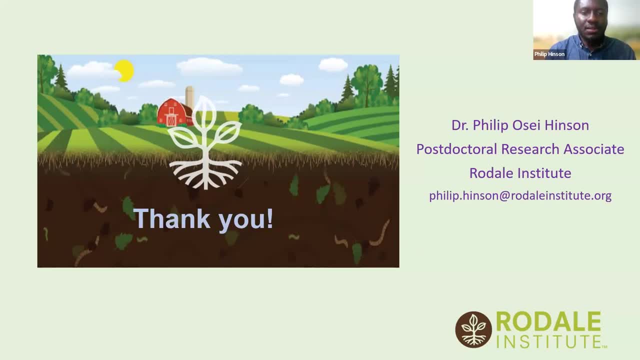 I have another question on: so dairy produces methane versus how much carbon is sequestered in the ground? Is it worth it? Yeah, this is a much difficult and complicated or complex question. It's hard to say. You know the global warming potential of methane is much higher than carbon dioxide. 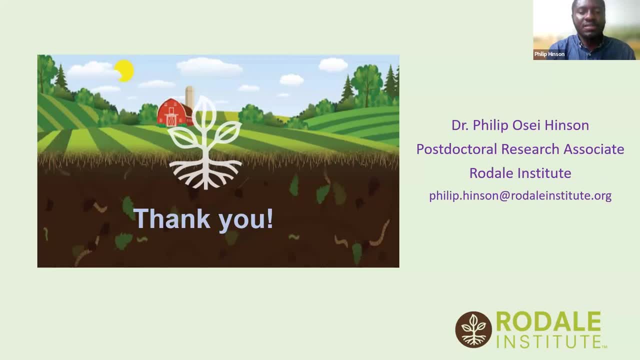 It's about 25 times higher than carbon dioxide, So it depends. The answer to this question is: it depends on how much methane you are producing and how much carbon dioxide you are able to sequester. So, like I said, or like I mentioned during my presentation, is the balance. 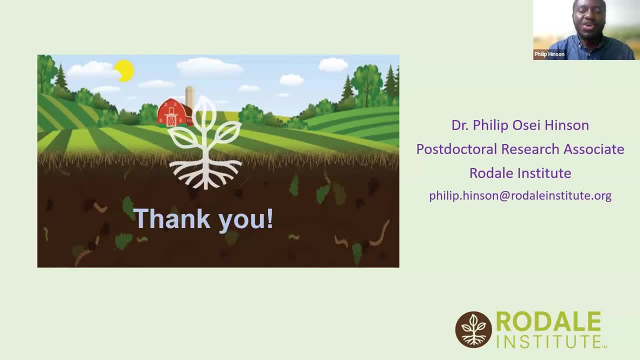 So is your inputs much, much higher than your outputs. That's what we need to reduce the effects of climate change or mitigate climate change. So, provided your inputs, which is When provided you have the ability to sequester or remove more carbon dioxide from the atmosphere.